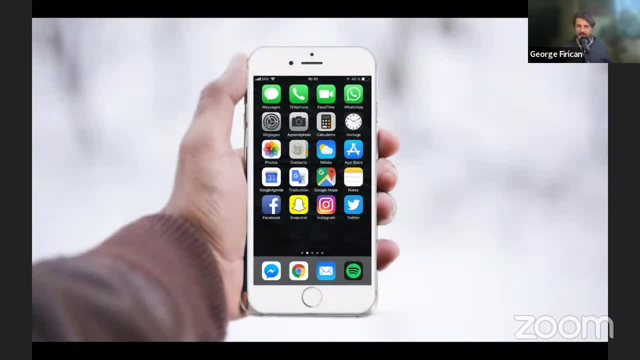 Well, you know, if we're just referencing our smartphones alone, I can tell you that there's about 40,000 apps that are added to the App Store every month, And that's just the App Store. really, That's a lot of apps getting added and refreshed. There's a lot of data that. 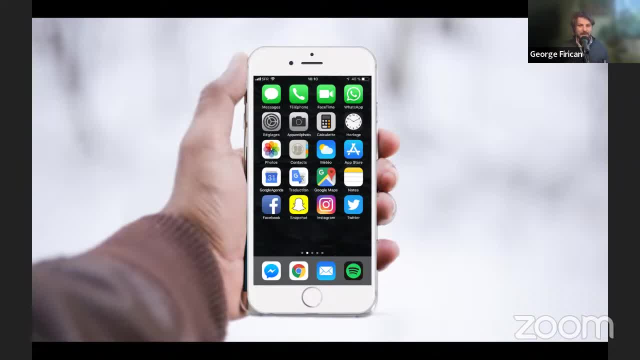 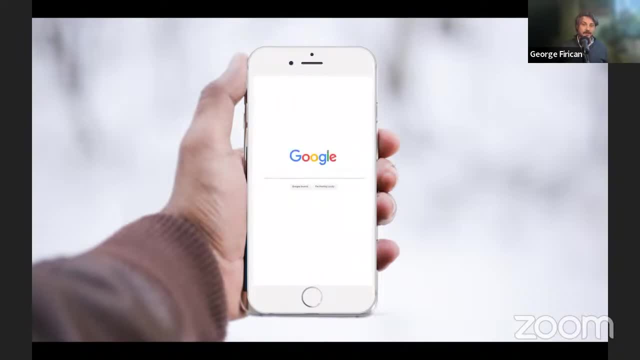 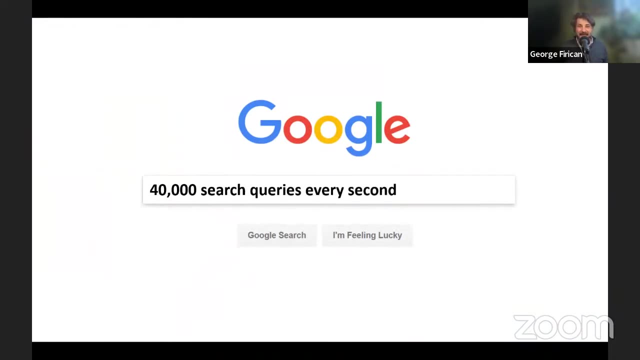 gets sent back and forth between the users and the data provider, the app provider too. Now, if we were to do a Google search right now, we would really be just one of 40,000 search queries happening every second. That's insane. That's huge. 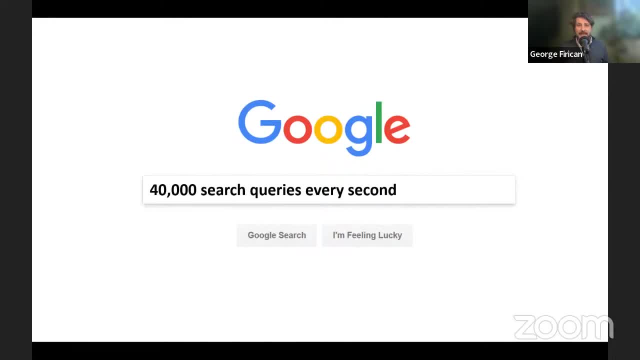 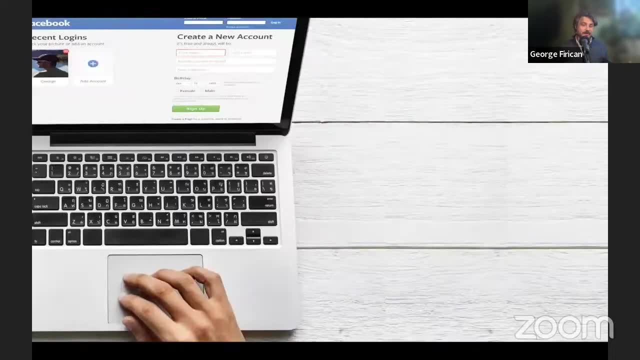 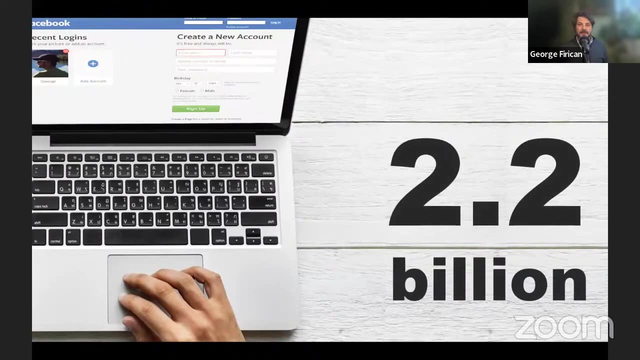 That's 5.5 billion Google searches happening every single day. That's big right. That's definitely big data. Well, Facebook can also give us an example of how big is big data. They have about 2.2 billion monthly active users. I know our CRM at university well. one of them really maybe. it's about, let's say, a million customers And monthly we have, let's say, 500. Unique users that are kind of accessing that CRM. I mean, compare 500 to 2.2 billion, That's. 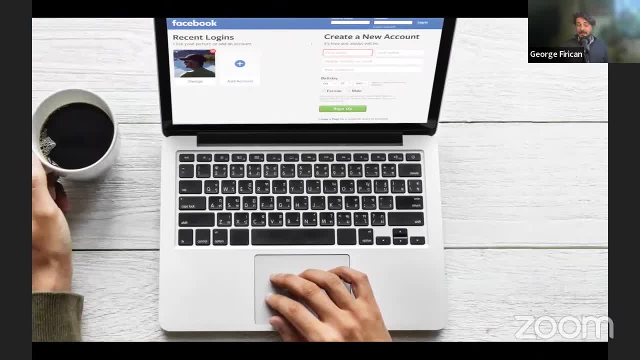 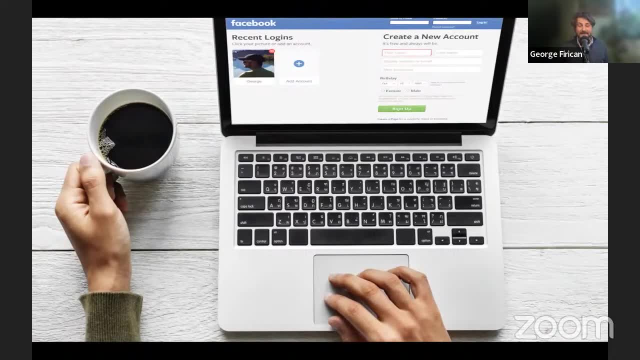 not that much of a comparison right Now. coincidentally, 2.2 billion is also how many cups of coffee are consumed every single day. That's a lot of coffee. I'm not doing my part today as I'm having my black tea, but I usually do enjoy my lattes, And I don't know which stats. 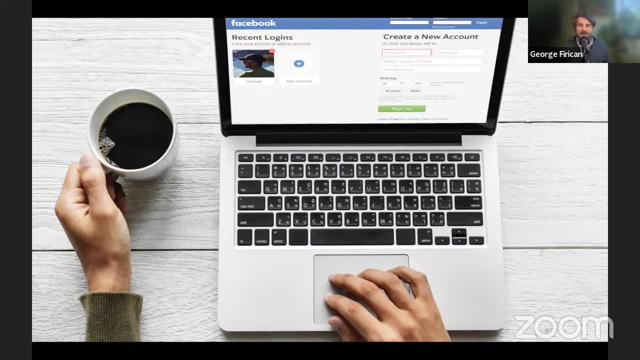 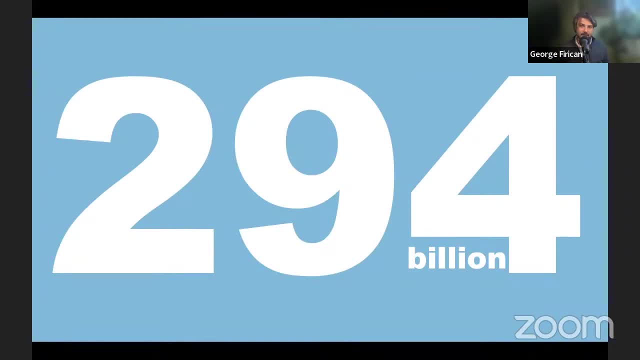 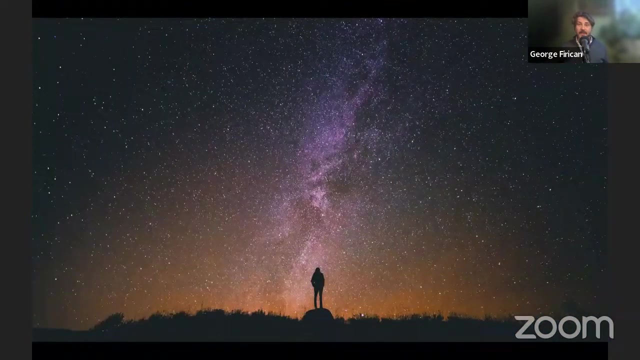 I'm more amazed by Probably the coffee Right. That's an insane number. If you're not convinced that big data is big, I'll give you another number. That number is 294 billion. 294 billion emails are being sent on a daily basis. To put it in perspective, our Milky Way galaxy has about 300 billion stars. 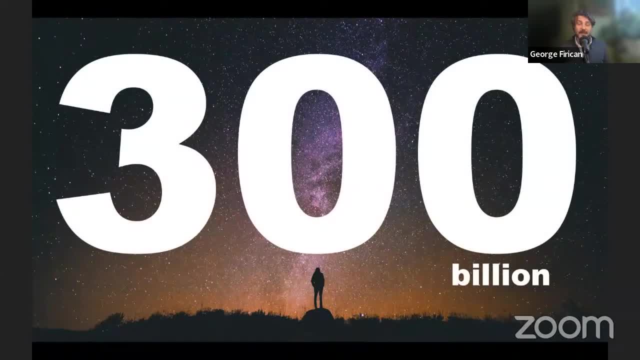 So that's a lot of emails, which is why I tell my boss whenever he's complaining that I don't answer my emails right on time. It's because we are getting a lot of emails altogether. So big data is big and that's kind of one of its characteristics. right, It's volume. 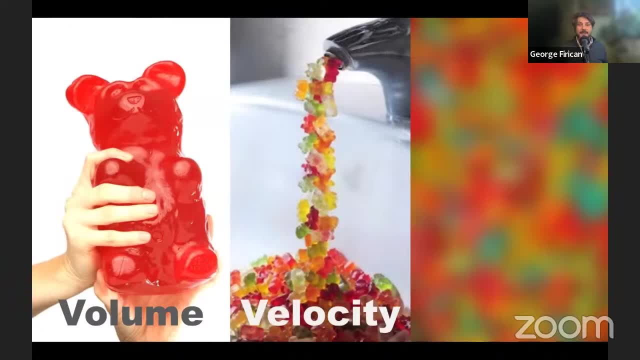 As we heard. it's also the velocity. you know the speed at which data gets created, consumed, processed. I mean 40,000 Google searches per second. There's 400 hours of YouTube videos added every minute. There's 2 billion Facebook messages sent every hour. still, 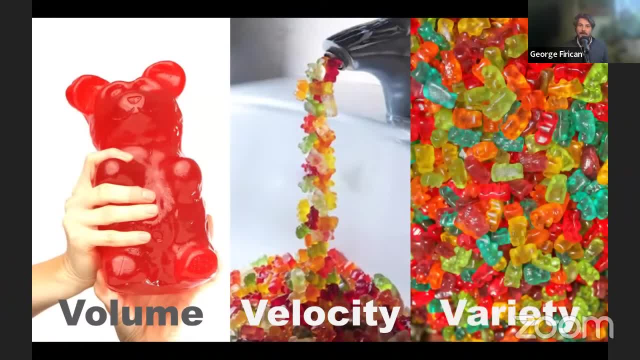 So that's a lot of emails And that's kind of one of its characteristics, right, It's volume, It's a high velocity. Big data is also quite varied. There are a lot of you know data types And sure about 90% of it is considered unstructured data, such as videos and audio. 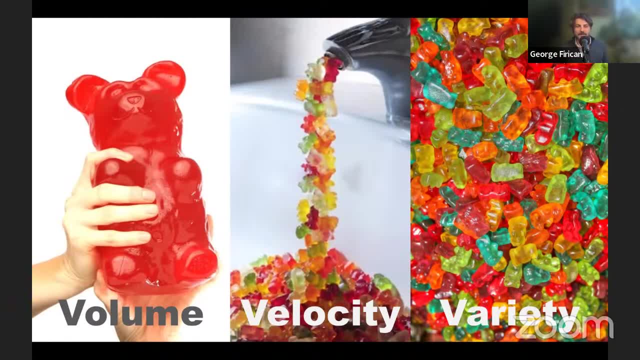 and photographs, texts, phone recordings and so forth and so on. The other 10% is usually semi-structured data, such as emails, or structured data such as financial transactions. So a lot of data types and data sources, a lot of variety. 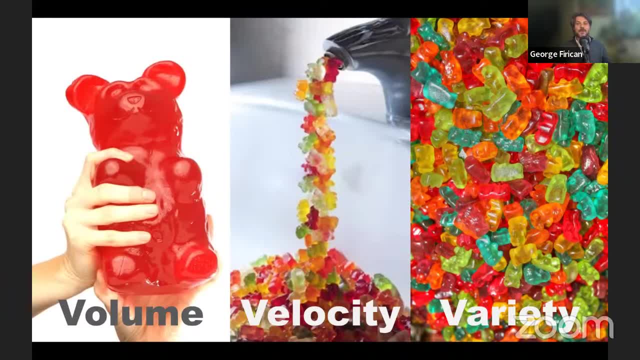 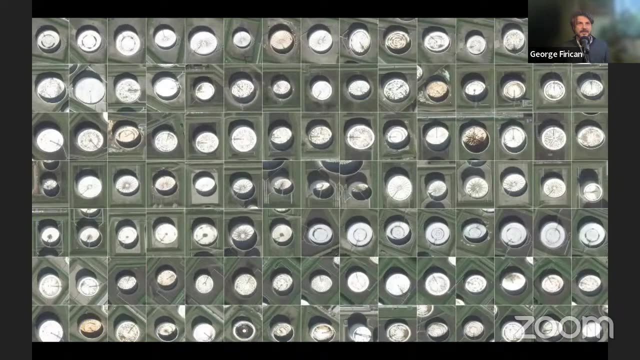 So these three characteristics are called the three Vs of big data, which I think a lot of us are familiar with. But now I want us to take a look at a couple of other big data examples which are a little bit different. Now I'll give you a second there to kind of think. 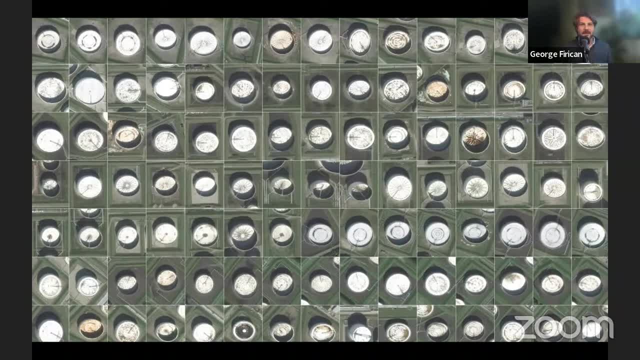 what are you looking at here? What do you think this is? If you have any thoughts on it, you know. please feel free to share in the comments for all of us to see. It's not really a trick question, but it does seem a little bit confusing. You know, I did see like wheels of cheese before. 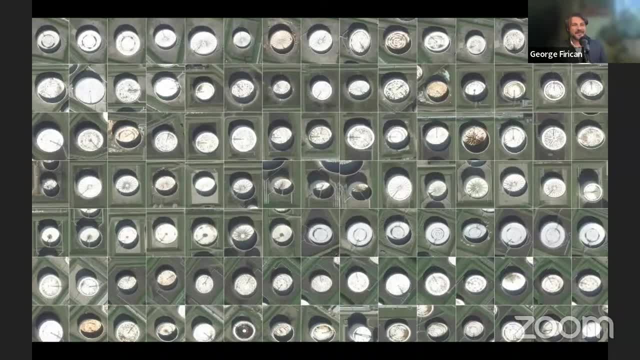 and a lot of crazy, crazy ideas, But you know it's up to your interpretation. That being said, I'll tell you really what we're looking at here. So this is a grid as we can see. It's a grid of satellite images, And each square depicts an oil tank just photographed. 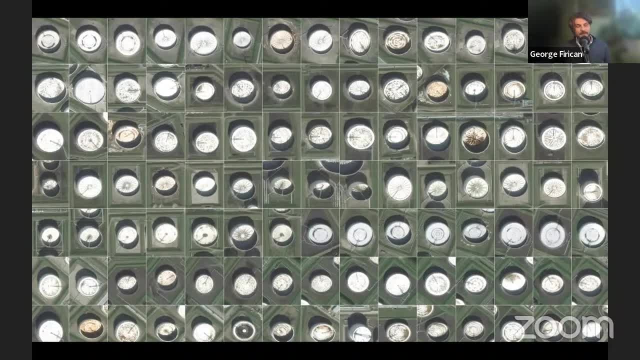 from above across the entire planet, And this is a grid of satellite images And each square depicts an oil tank just photographed from above across multiple weeks. Why are we seeing this grid here? You see, a while ago the US wanted to better estimate. 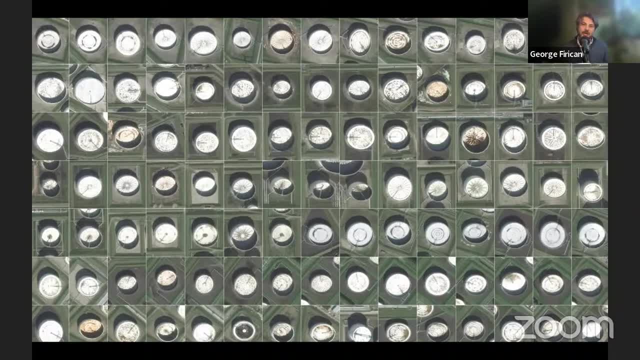 China's oil supply And by looking at the changes in the shadows cast by the floating roofs of oil tanks, analysts could estimate how much oil was available in all the tanks. it was monitoring right. So as the oil was being depleted from this tank, this cylindrical tank, its roof was dropping. 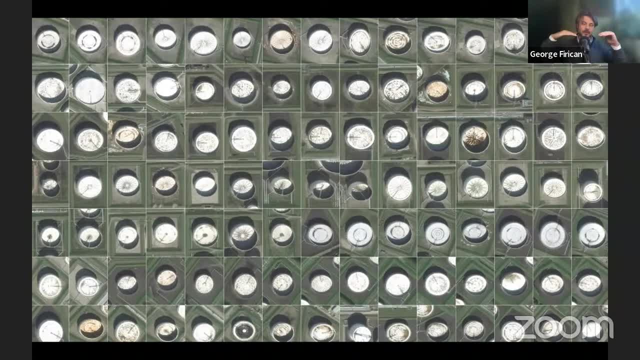 and the walls of the tank was casting a different shadow onto the roof, So we can see here different shadows at the same time of day, And that's how they were able to better estimate China's oil supply. And a fun fact, from what I understood, 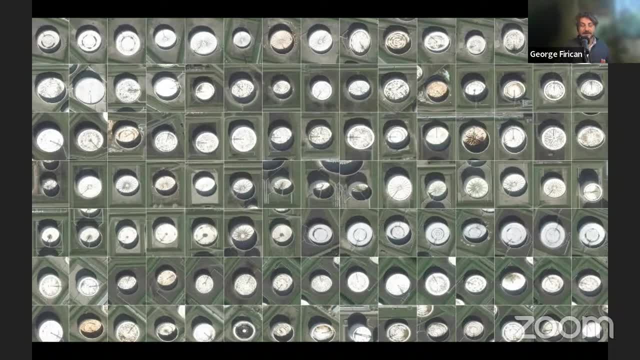 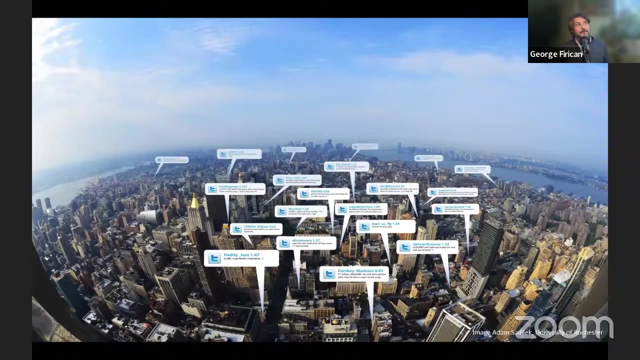 the estimate that was done by the American analyst was really higher than the official declared value by China. But that's neither here or there, It's just really an interesting example Of big data. I'll give you another one. This one comes from a research team from the University of Rochester. 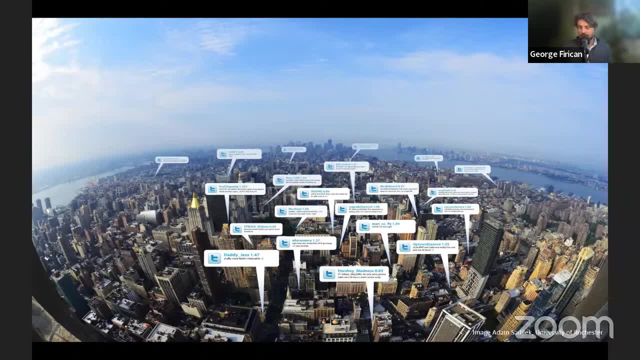 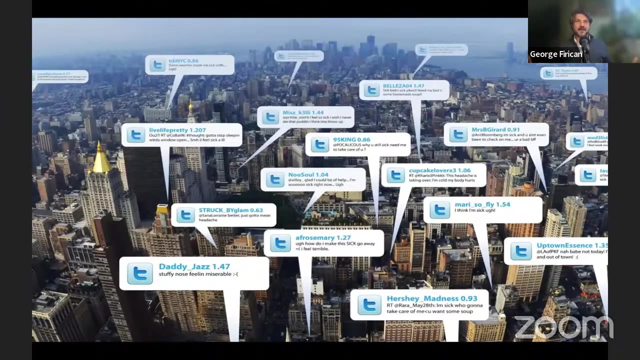 And they've created an algorithm that could spot flu trends and make predictions based on keywords in publicly available geotagged tweets. So let's zoom in here a little bit. This is a view from New York, with all these fictional tweets that we're seeing. you know people saying 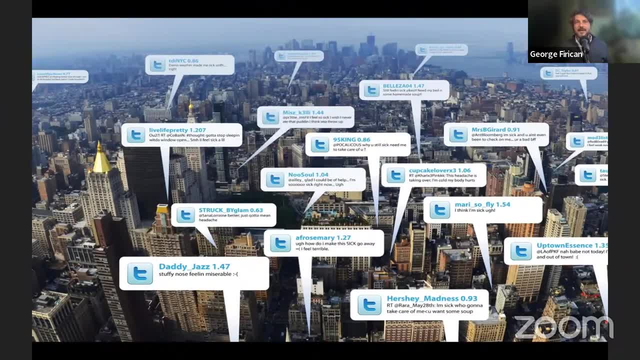 oh, I'm so sick. I feel like I'm, I'm, I'm, I'm feeling miserable. I need some chicken soup. Oh, I need to be in bed, And somebody please take care of the sniffles, So forth. 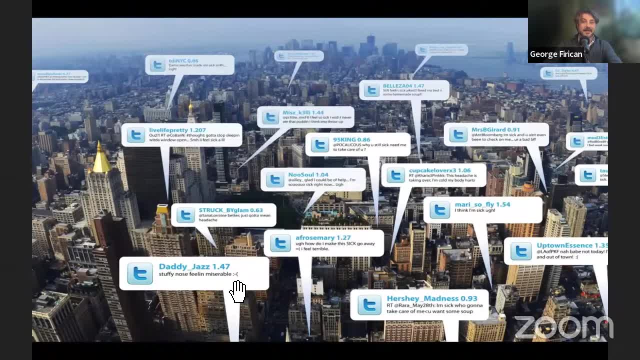 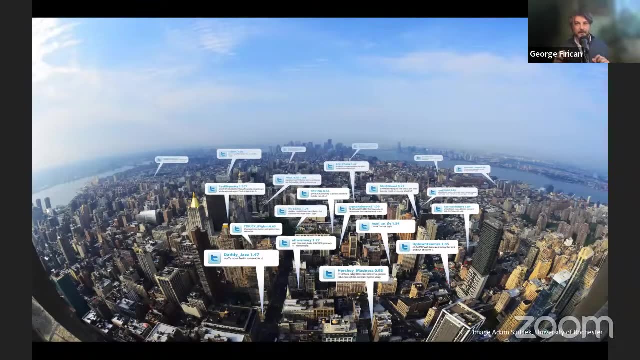 That's one A lot of different tweets, And the cool thing is that the algorithm could track the spread of flu and predict which users were going to get sick next. Pretty cool, right As you can imagine, I think this was also used for for COVID afterwards. 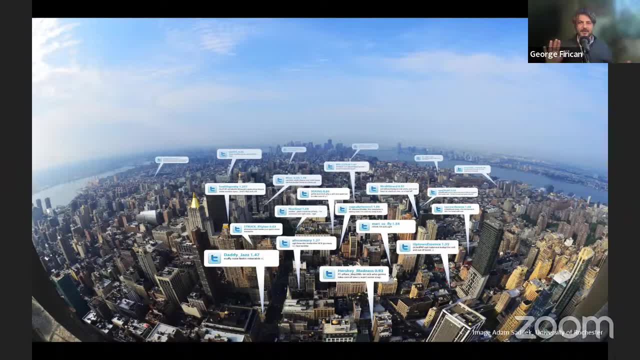 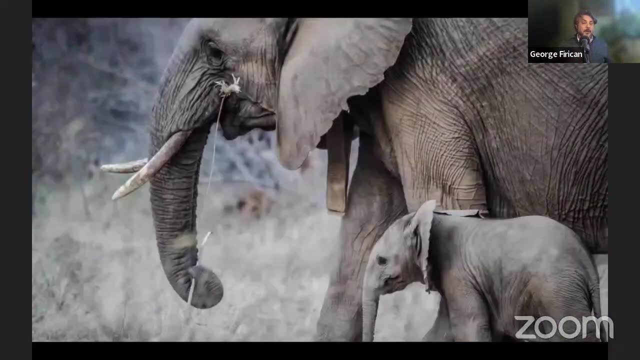 But I just know what the data and the analysis that was done based on the flu predictions. Now, both of these data sources that we saw, they're unconventional for sure, but they both pose big, complex problems. So both of the data sets that we saw, 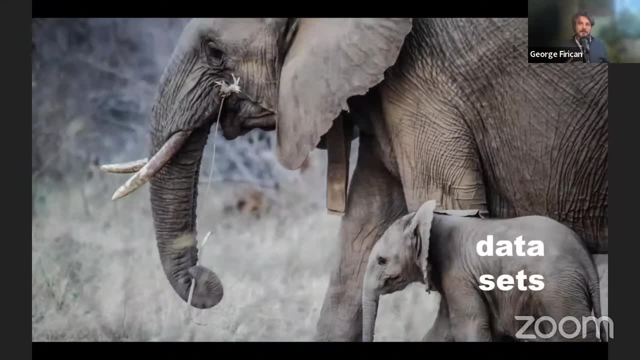 they're actually not that big. You know there are only a few. you know tens of thousands or maybe even hundreds of thousands of records in each one of these data sets, In a way kind of similar to the data that a lot of you know, smaller organizations. 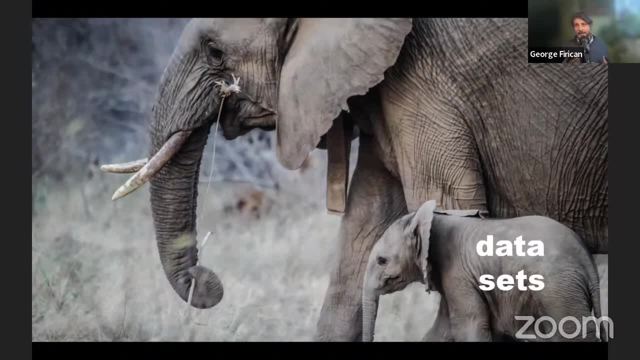 medium-sized organizations are working with. You know we all say that we're not necessarily working with big data in our job, even as data scientists, data analysts. A lot of times we're not working really with big data. So you know, if you think about it. 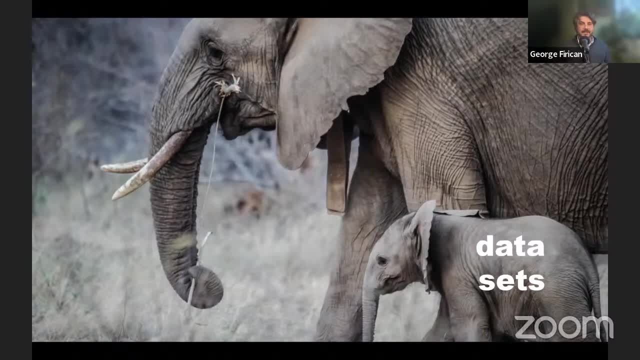 these two data sets as well. they don't really have a lot of different types of data. You know, there's not that much of a variety. It's kind of tech-oriented and it's kind of tech-oriented and it's kind of tech-oriented. 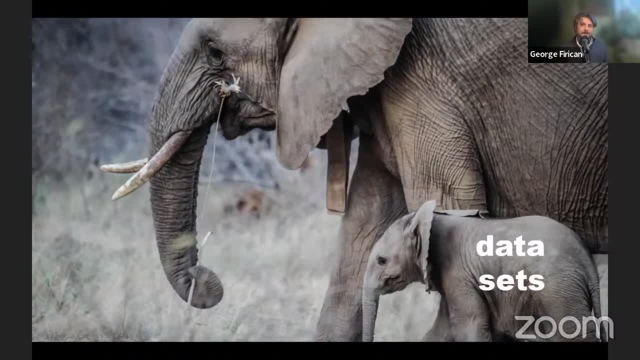 and images and a couple of data dictionaries attached to each one. As for the velocity, well, the data doesn't need to get processed and analyzed very fast. I mean, let's take the tweets, for example. Even if those get produced and outputted every second, the algorithm doesn't. 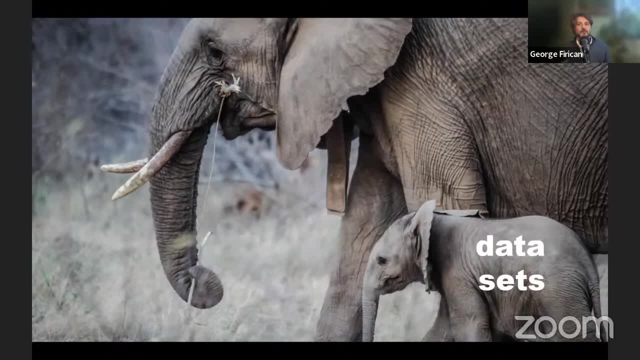 need to process them right away. It could actually wait a day or even a week, as it could still look at the timestamps and process it later, As with the satellite images. yeah, that's definitely not a high velocity there. The photographs are being taken every few weeks, every few days. 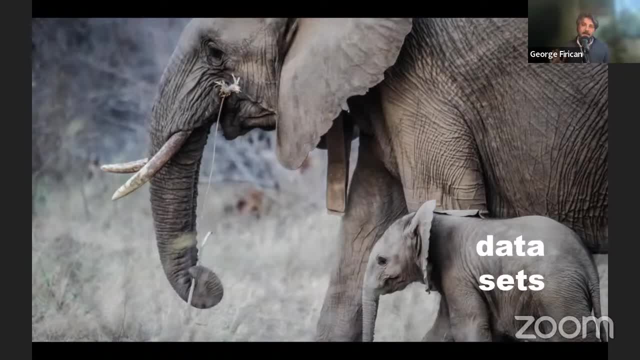 It does take quite a bit of time. The point is, though, that both of these data sets- and, I think, including our own, including a lot of the data sets that we're working with well, they still pose big, complex problems. I mean, it's not easy to estimate China's oil supply. 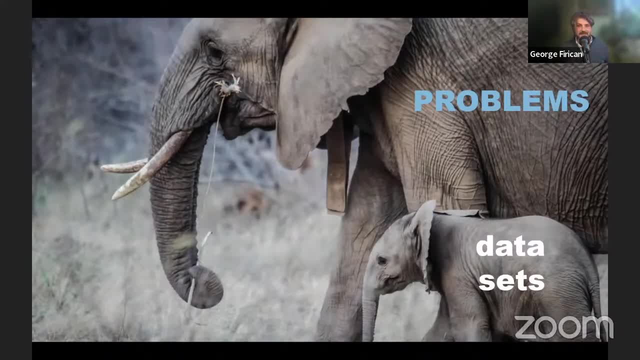 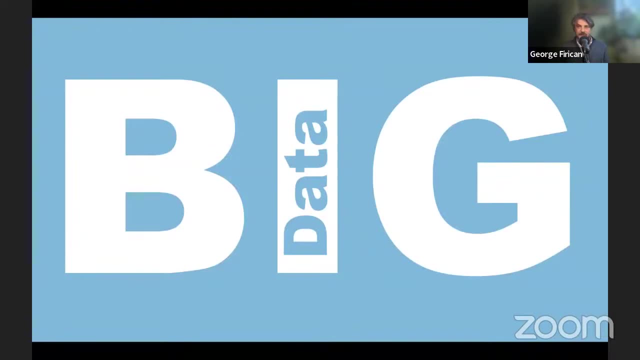 right. So what's my point? Well, we know so far that big data is characterized by its big volume. you know velocity, variety, But big data as a term, I think, can actually be a little bit misleading, As it's making us focus on its size. we kind of miss the most important nature of the 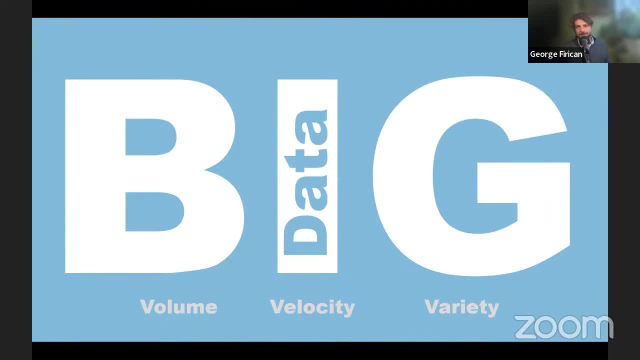 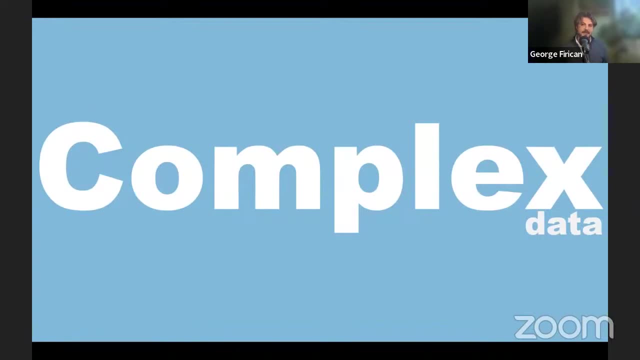 medium, And that's the complexity. So let's push big data out of the way and think of it as complex data instead, Because this complexity is not only due to its size- you know, velocity, variety- but other factors as well, And all these other factors, like they, add up to what I call the 10 V's of big data. 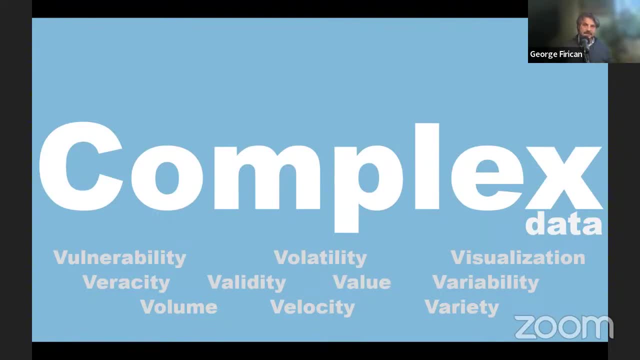 or complex data. So, again, let's throw big data as a you know, big size concept out of our mind, because it's not the only important thing When it comes to big data. So let's try and uncover some of these other V's and see what. 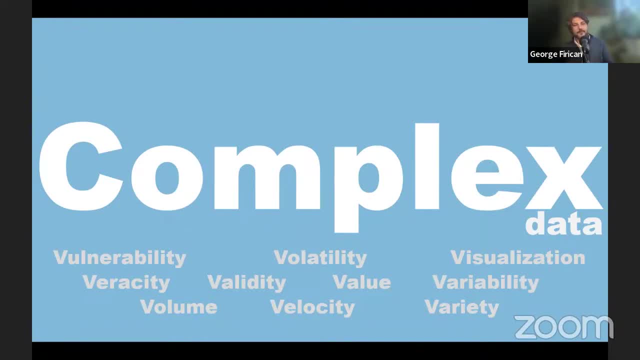 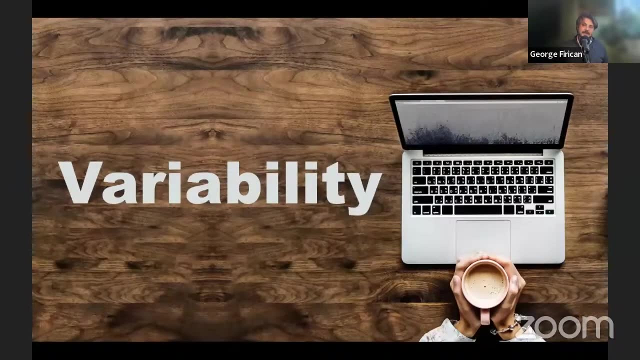 they stand out for and how they are a characteristic for big data. So the first one is variability. Variability in a big data's context really refers to a few different things. So let's see what we mean by variability. It's often confused with variety and it's not the same thing. 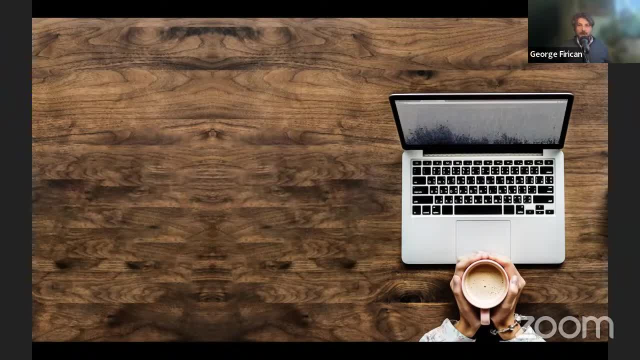 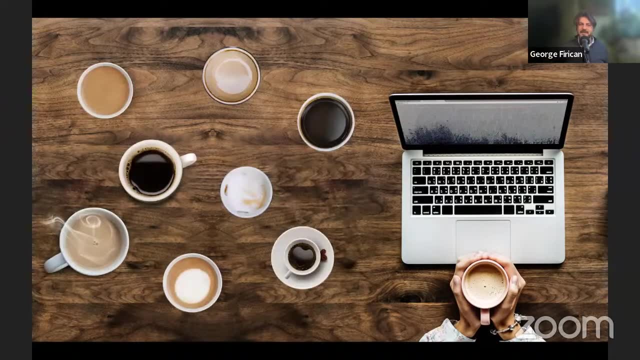 Let's say, let's say here that you have a coffee shop that sells all these different types of coffee. You have your Americano, you have your latte, your espresso, your London Fog cappuccinos- what have you? 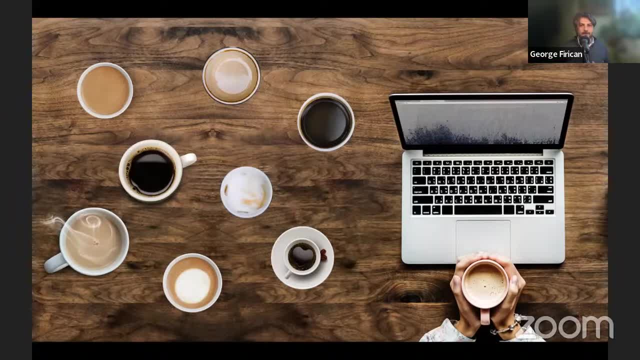 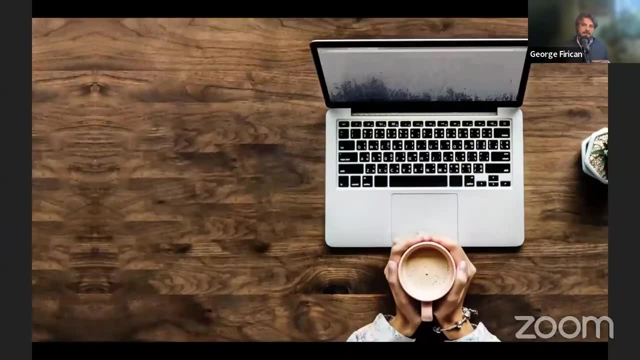 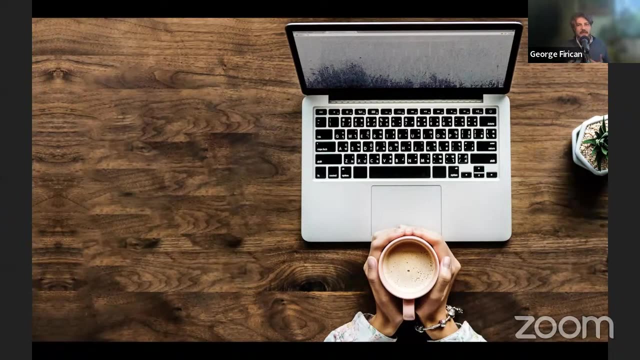 Now, this represents variety. There's a variety in offerings. I imagine that you go to the coffee shop three days in a row and every single day, every time, you buy the same type of coffee- In my case it's always a latte- But each day this latte tastes and smells differently. That's variability. 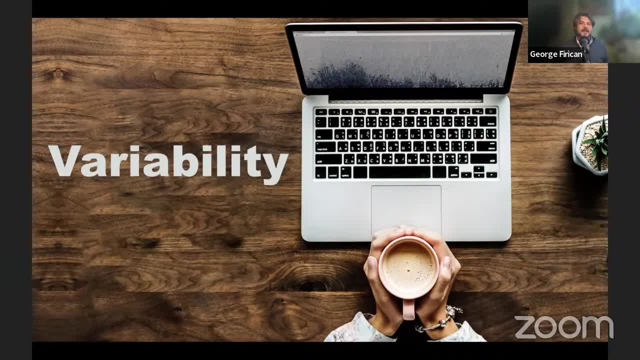 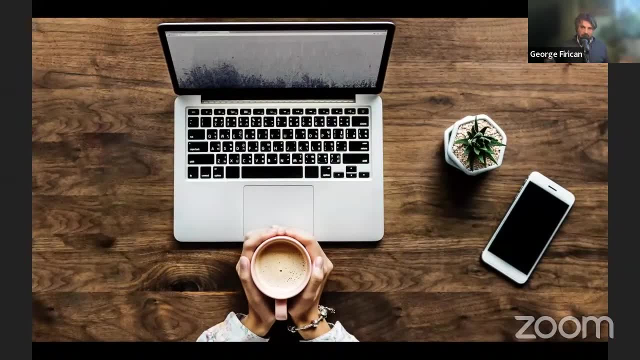 Translating it to data, it really reflects the number of inconsistencies that we find in data. As I mentioned, variability refers to again a few different things. Brian Hopkins actually, who's a first year principal analyst, defines variability as the variance in meaning, in lack of meaning. 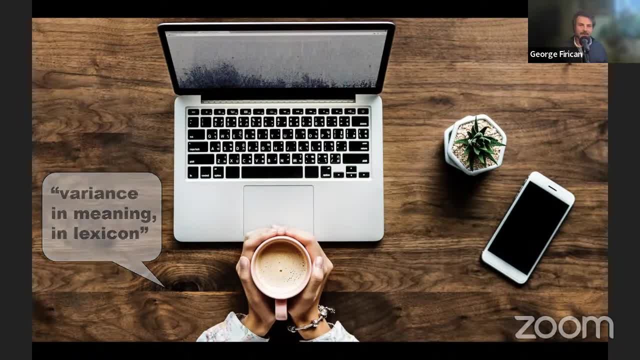 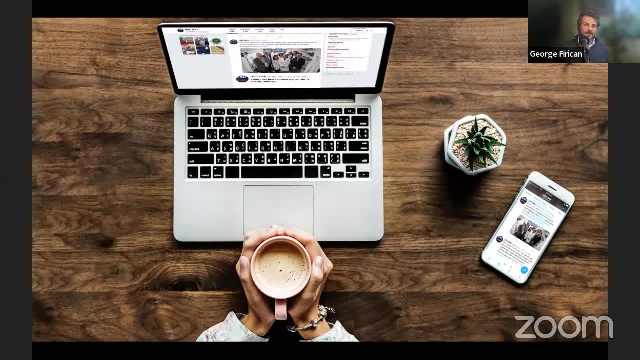 The variance in meaning in lexicon. What does that mean? Well, let's take a look at a Twitter feed as an example. This one is from my university, where I work at Now. variability becomes very relevant in performing sentiment analysis, because the meaning of a word 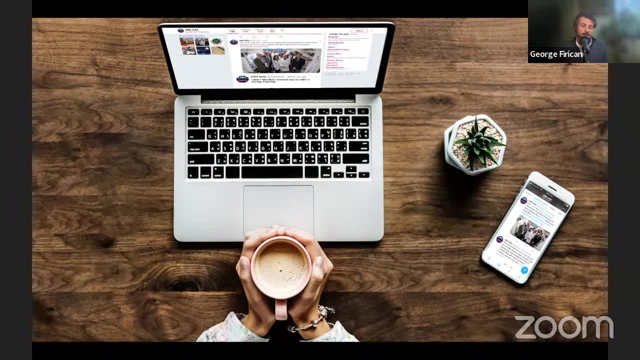 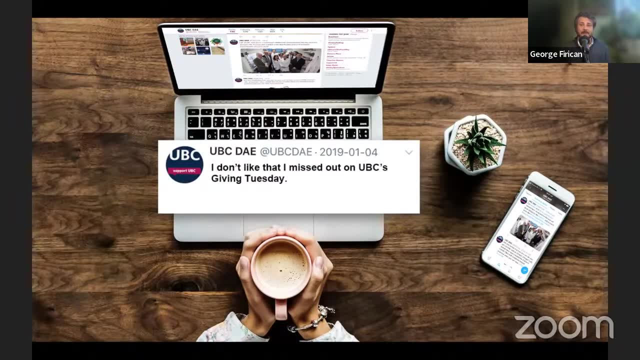 or a group of words changes especially depending on the context. So an example: let's say you know there's this tweet that says: I don't like that. I missed on. you know UBC's Giving Tuesday, which is kind of this, like you know, one day opportunity to donate via your text and all this stuff. 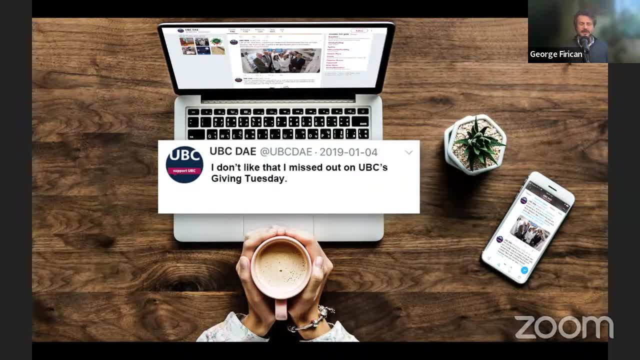 There's different methods and celebrations and the university trying to raise funds for its students and research and student awards and whatnot. Now, reading this out, I don't like that. I missed out on UBC's Giving Tuesday. It's obviously, you know, a positive thing, but the algorithm might see it as a negative one, right? 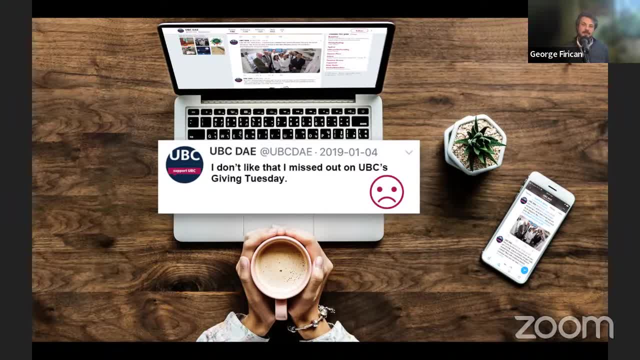 Because to perform proper sentimental analysis, the algorithm really needs to be able to understand the context and to be able to decipher the exact meaning of the words in that context, And this is still very difficult to do. Yes, things are improving, for sure on this. 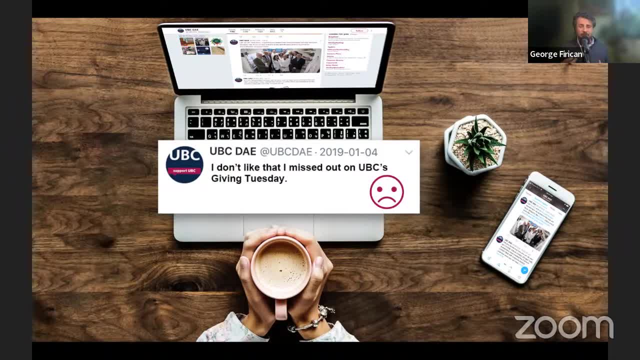 There's more and more dictionaries out there and there's, you know, a better AI that's being developed, But it's still- It's still not as accurate as a human's- I guess, interpretation of reading this and understanding all the context behind it. 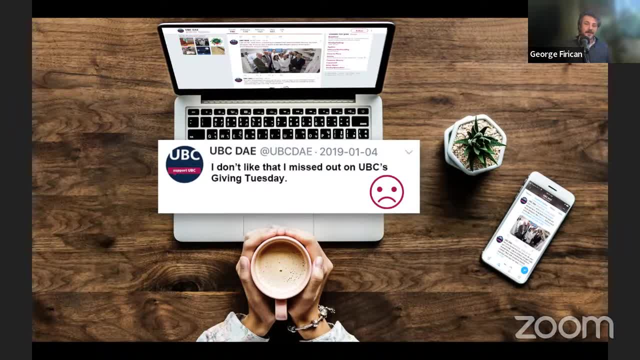 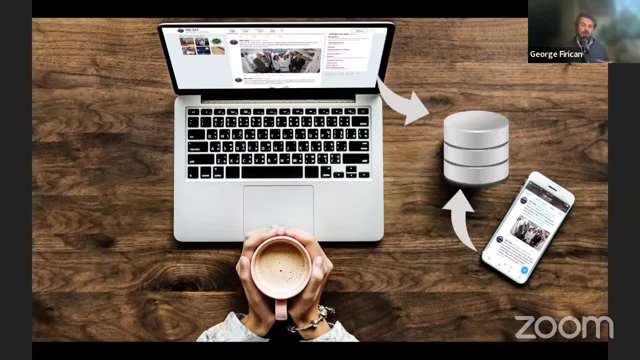 So it's still a very difficult thing to do. Variability also refers to the inconsistent speed at which data is loaded into your- you know- data stores and your databases, So there's definitely some variability there as well that can pose different challenges. 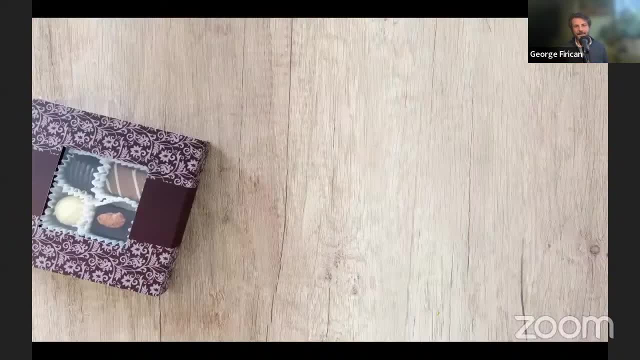 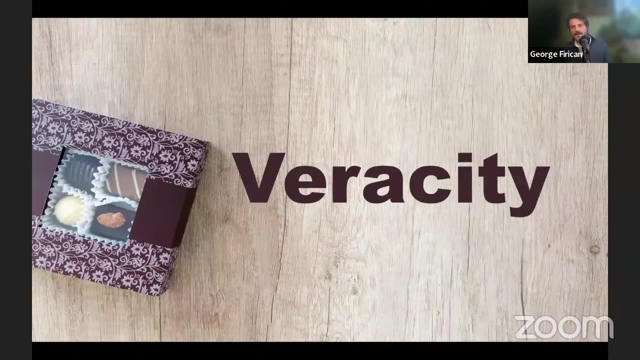 Especially from a Data engineering perspective. Next one. Next one is veracity. Veracity refers more to the confidence or trust in data based on the provenance or the reliability of the data source. You know its context and how meaningful it is to the analysis based on it. 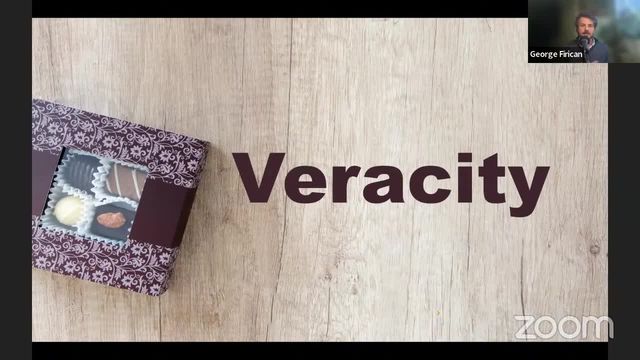 Let's think about it this way: When you get a box of chocolates, how do you estimate how good it is before actually tasting it? You know, maybe you look where it was made, but what shop, And so on? right, So I'm Romanian originally, hence the accent. 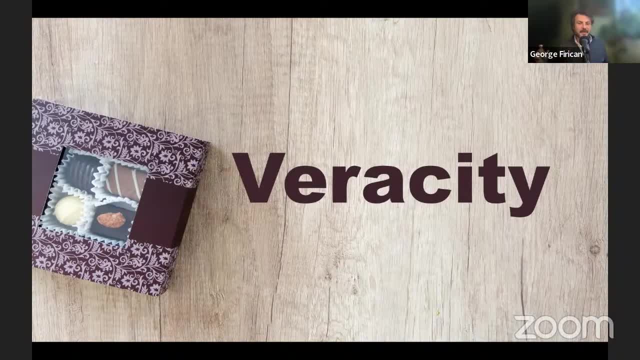 If I were to get, let's say, a box of chocolates and it says made in Romania- I don't know, Romania is not really known for making chocolate, but if I would see it made in, you know, Switzerland, like Swiss chocolate, I'm like, oh yeah, give me that. 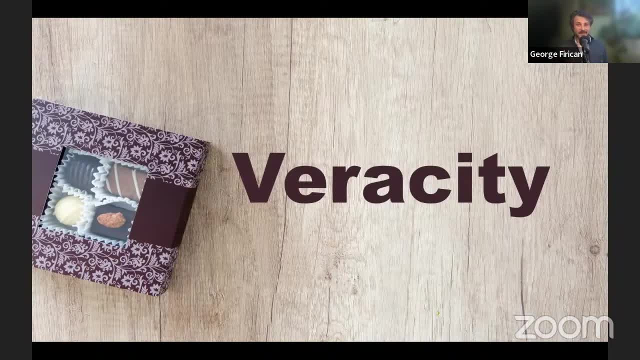 I'll open it and eat it up right away. So you know, that's my way of kind of gauging its veracity. And, by the way, Romania does not have bad chocolate. It's actually pretty good, But I think Swiss chocolate is probably one of the best ones out there. 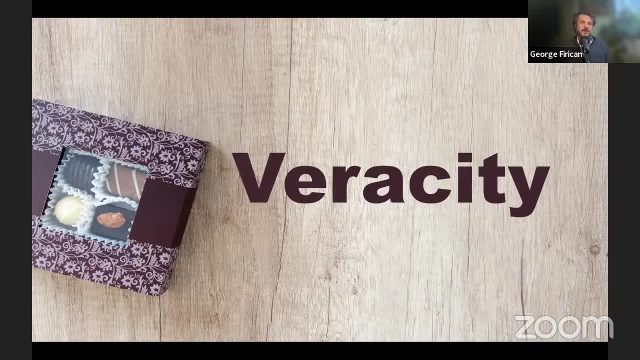 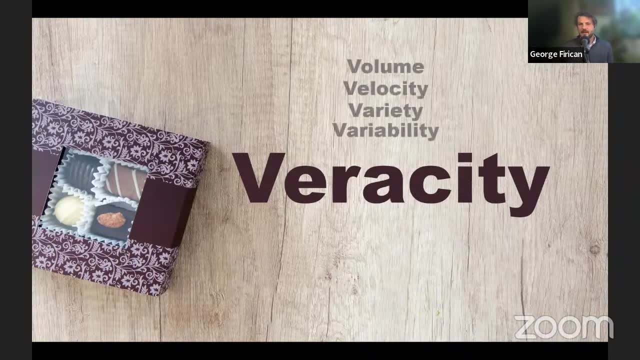 So one thing that I do want to mention about veracity is that it's kind of one of the unfortunate characteristics, let's say, of big data, Because as any or all of these properties increase, so the volume, velocity, variety, variability, as all of these go up, the veracity or the confidence. 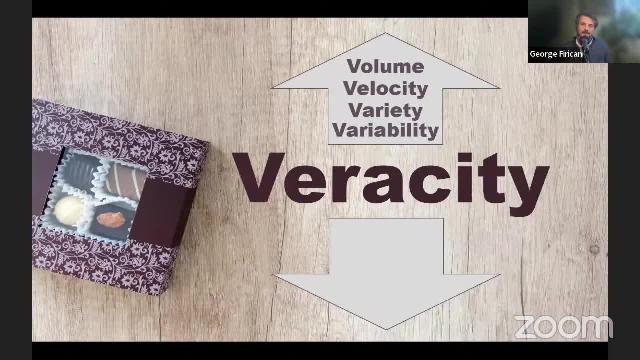 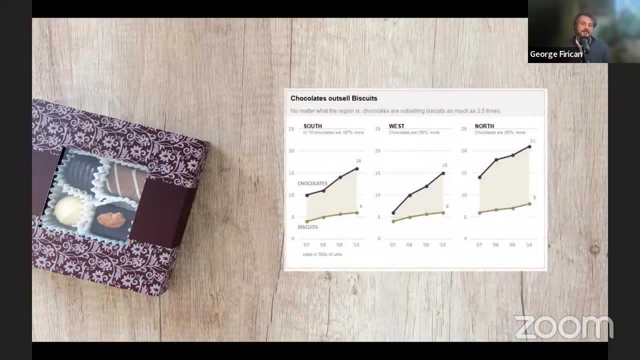 or trust in data tends to drop, And again, unfortunate. So, for example, let's consider a data set of stats on what desserts people purchase at restaurants and shops, and you know these items prices over four years. We might ask ourselves: OK, well, who created this data source? 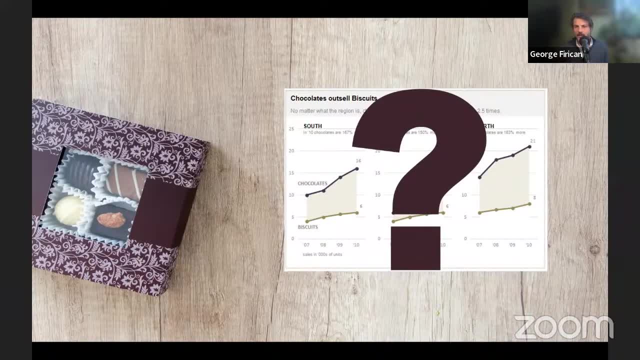 What methodology did they follow in collecting the data? Were only certain cuisines or certain types of restaurants being included? You know certain types of food. You know certain types of desserts. Did a data creator summarize the information? Has the information been edited, ultra-modified by anybody else in the process? 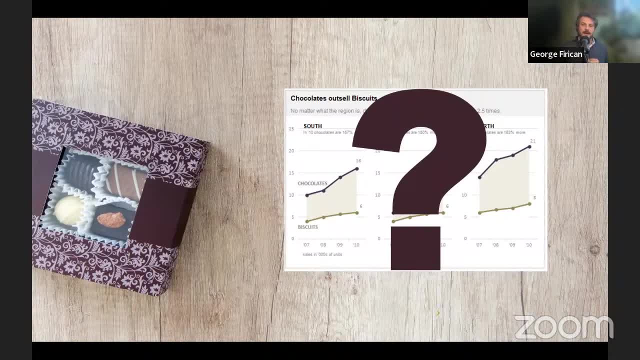 And as data scientists, as data analysts, we need to ask these questions And it's necessary to get those answers in order to determine the veracity of this data, of this information, And knowledge of data's veracity in turn helps us better understand the risks of data loss. 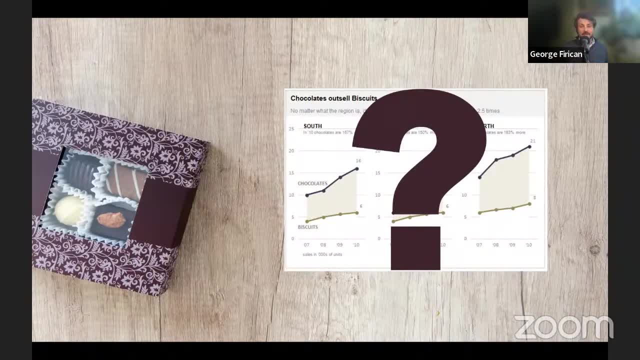 And knowledge of data's veracity in turn helps us better understand the risks associated with analysis and business decisions based on you know, a particular data set. So let's always remember and make sure that we're kind of checking all these boxes for these questions. 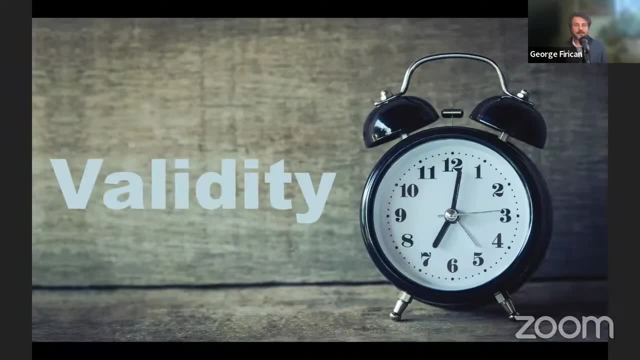 Validity, Kind of similar to veracity. Validity refers to how accurate and correct the data is for its intended use. For example, this watch you know works well. Probably It was probably not accurate to the millisecond. So let's say we're looking at registered charity data from the IRS. 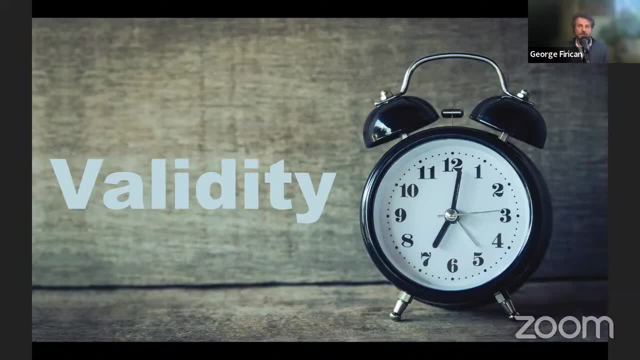 And in that main column we can find a list of names or job titles or even emails of those you know, charities' contact. Now they're all accurate contact information, But not if you're looking for the exact Names of the individuals. 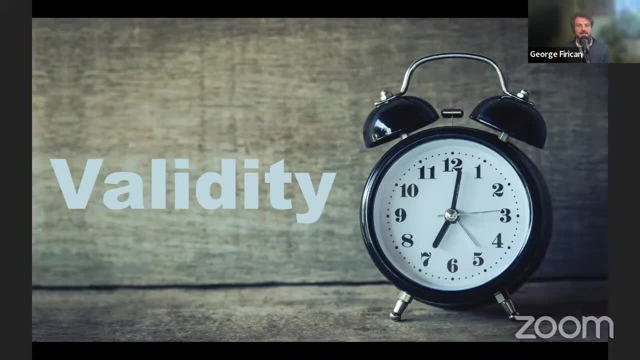 Sometimes in that list of names we're actually again seeing the job title instead: director of finance, Or we're seeing the like the finance at, you know, the gatesfoundationcom. So sure it's accurate. 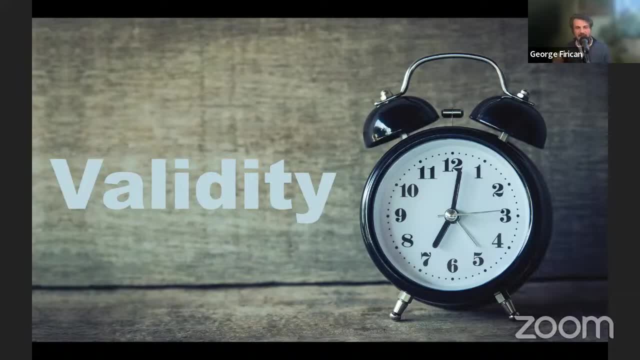 But not if we're looking for the names of those individuals instead. So, according to Forbes, As you're well aware of, an estimated 60% of a data scientist's time is spent cleansing data before being able to do any analysis. And, as data scientists, data analysts again, this is a big pain point for you. 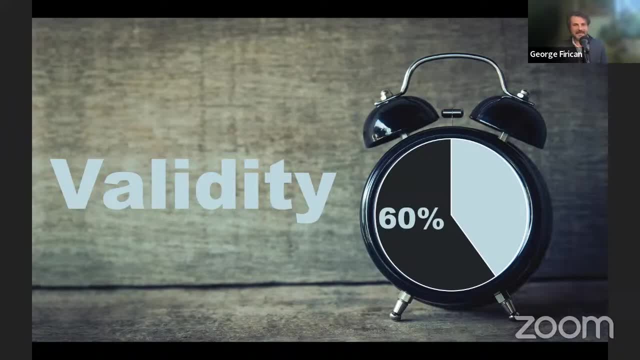 For all of us. really, We don't want to spend time cleansing this data, We just want to work and do our stuff there. We want to. you know, go and do what we're paid to do. Yeah, Obviously, the benefit of you know from. 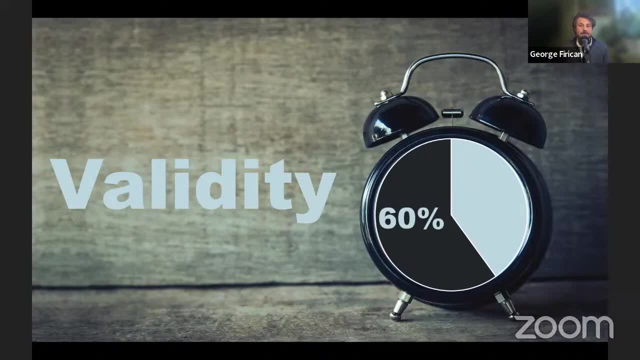 From big data analytics is only as good as its underlying data. So you need to adopt good data governance practices, in my opinion, to ensure consistent data quality and common definitions And described and understood metadata and so forth and so on, But that's another topic for another day. 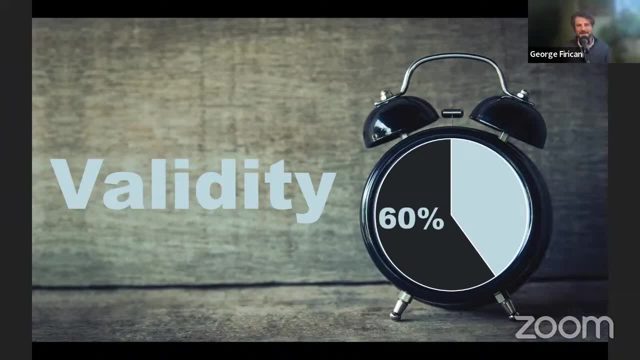 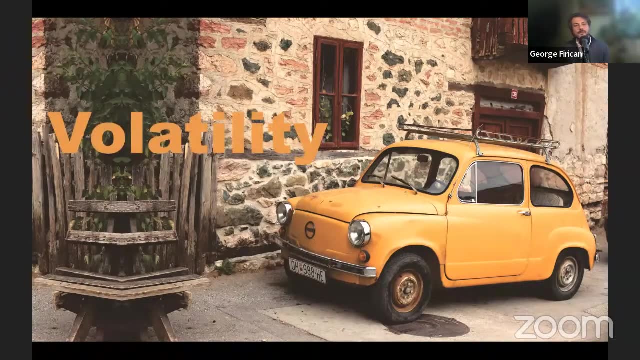 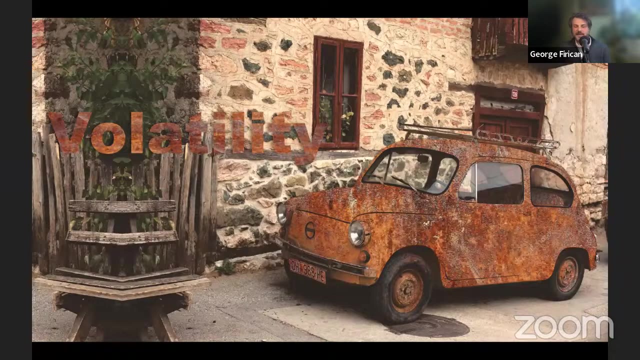 That's one of my specialties, by the way- data governance, So I could talk about that for hours. Volatility- So volatility is really referring to how old Your data needs to be before it's really being considered irrelevant, historic or just not useful any longer. 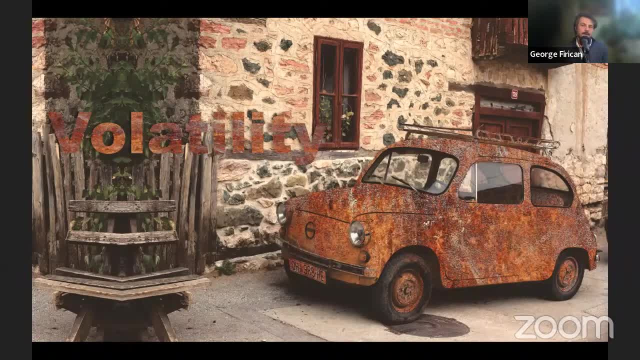 You know how long does data need to be kept for? You now need to kind of establish rules for data currency and availability, as well as ensure rapid retrieval of information when it is required. And you also need to think of it as well. 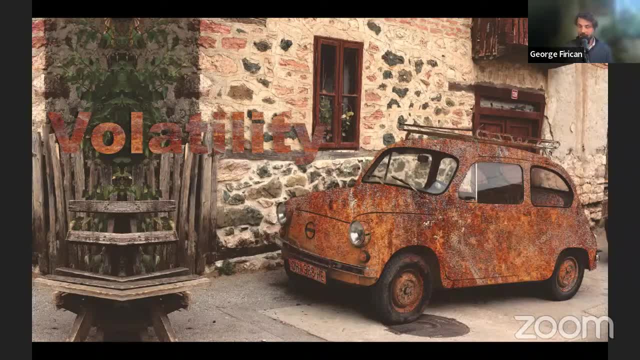 Okay, Well, it's the data. Is the data old enough, Or is the data too old to be considered for the analysis that I'm doing? Or do we actually need to have that retention piece put in place to kind of try and get rid of it, try and archive it? 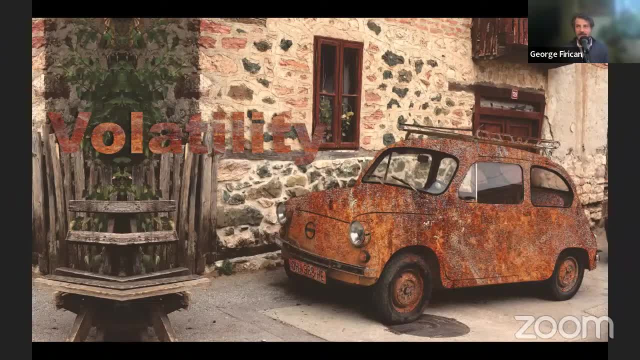 Otherwise, if it's not used, it sort of transforms into what I call dark data. It's just there for just in case you know we're hoarding it, But in doing so it can open a whole can of worms really. 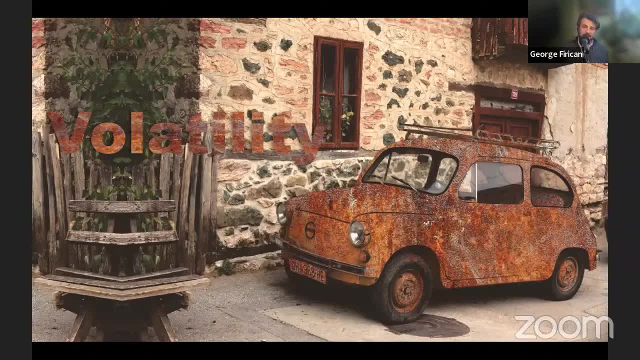 So make sure that You know all of these processes are kind of tied to your business needs And just you know, make sure there's something implemented there. I guess that's more for the data governance group, data management, even data engineers to help out with. 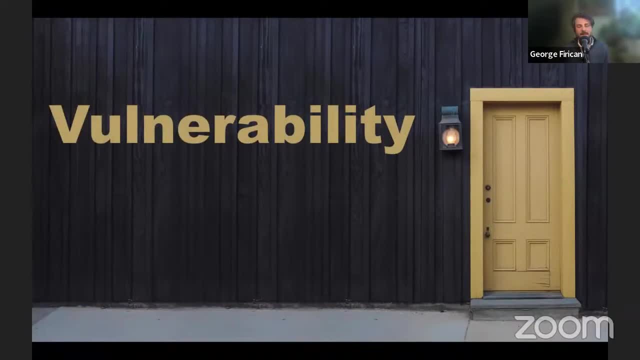 Vulnerability. That's another important V associated with big data. You know, as we saw from the oil tanks example, right, this complex data can really open some vulnerabilities. In the case, it opened some vulnerabilities within, you know, China. 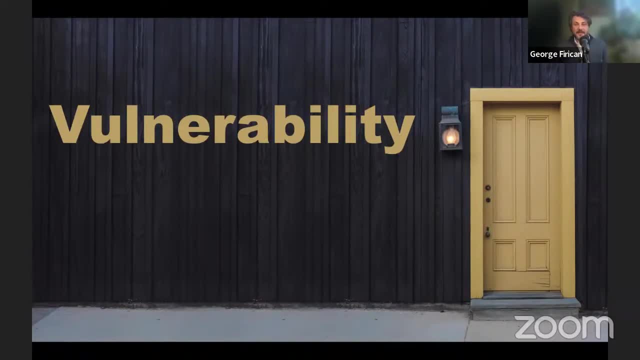 So different types of publicly available data about the same individual can actually reveal private information. You know, if you collate, you know photos and Twitter feeds and email addresses and so forth, like even in that example, with the tweets that, yes, we're sharing the fact that, hey, I need some chicken soup. I have the sniffles. 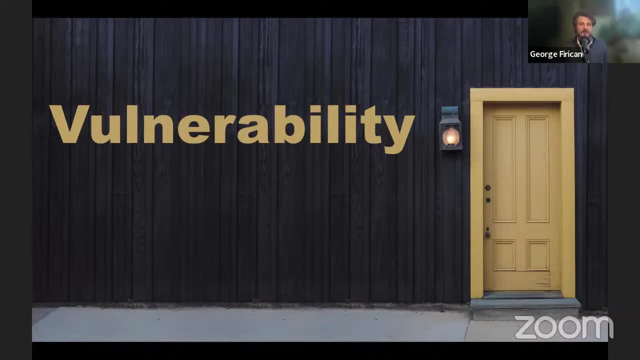 that can reveal some private personal information And maybe just tied to a Twitter name doesn't mean anything. But then if you're collating it with a bunch of other stuff, that where it's considered public information, we can actually find a lot of details about that one individual that maybe that one individual is not even aware of. 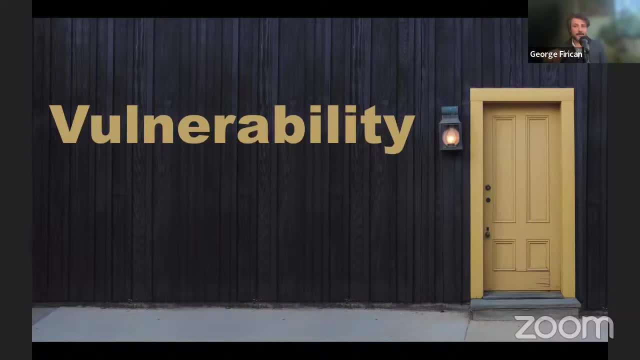 So you know, especially public information about the context of the individual, such as, let's say, census information on a neighborhood. Yeah, You can definitely discover a lot of more things about that. So there's always some ethical considerations to make. 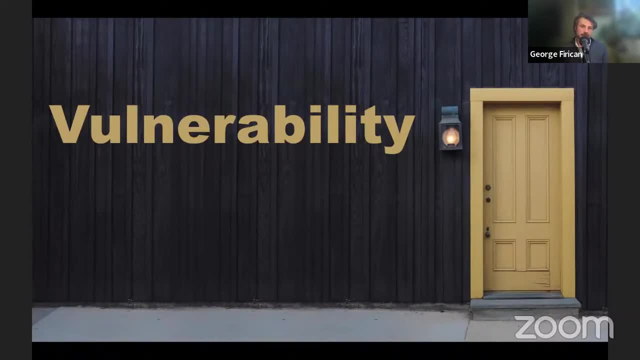 So big data brings new, you know, security concerns. Not surprisingly, one of the rationales for resistance to the use of big data in some organizations is concern over privacy, And there are a lot of companies that are especially sensitive to the perception that they will use, you know. 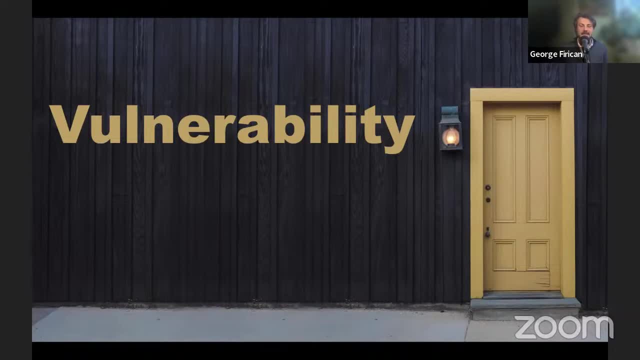 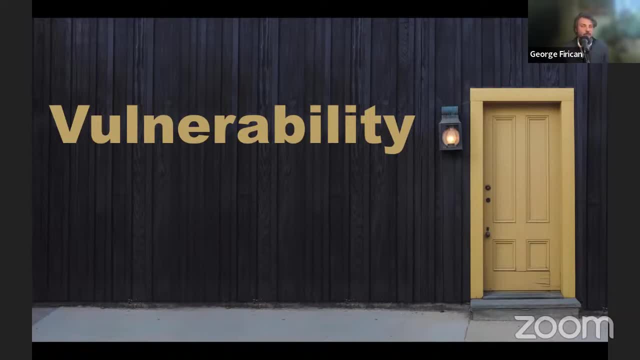 You know, without a data-driven targeting consumers and customers kind of wade through random advertising that offers them all the you know little benefit for their valuable time, right? That's. that's why now there's this trend to have all this personalized content. 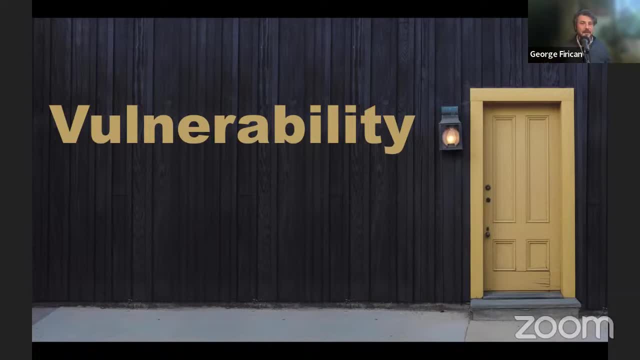 And yes, there's. there's a lot of other considerations around that too, But that that brings me to the point vulnerability. vulnerability because it can open up that, that data security door, And we don't want that. We, we definitely don't want that, especially with big data, and not just because of the size. 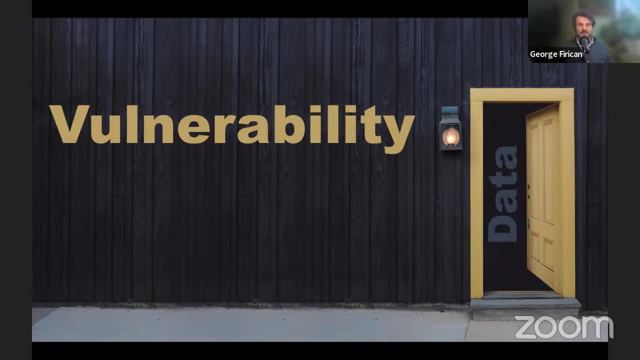 I mean, after all, data breach with big data is kind of a big breach, But also because, if you have multiple data integrations, a data breach into one can open a vulnerability into another and even into your main database as a result. 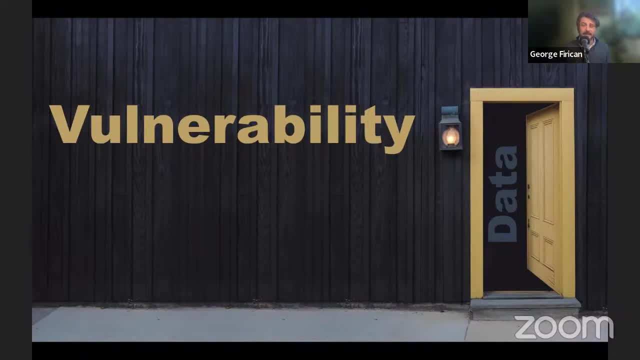 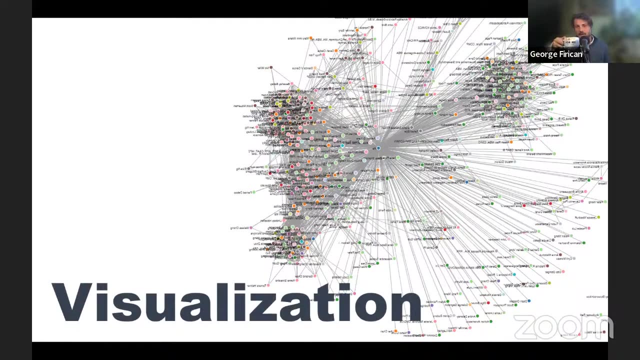 That's not something that we want, So this is a V that we need to be very careful about. Visualization: This is another characteristic of big data: Just how challenging It is to visualize it. I mean, current big data visualization tools really face some technical challenges due to limitations of in memory technology and for scalability, functionality, response time. 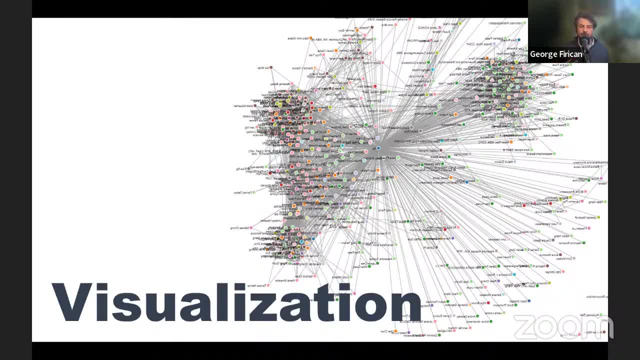 And, yes, these are improving where we're having better, better solutions and tools. you know, almost every month really, Um, the fact of the matter is, you can't really rely on traditional graphs when trying to plot a billion data points, right? 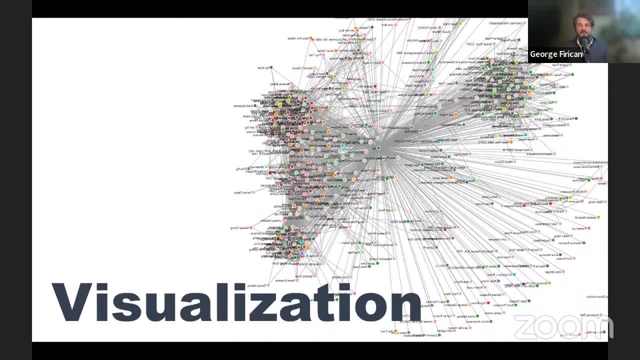 Uh, with, You know, having visualizations that contain dozens of variables and parameters. This is really a far cry from the X and Y um variables of your standard bar chart right, And finding a way to present this information that makes the finding clear is one of the challenges of big data. 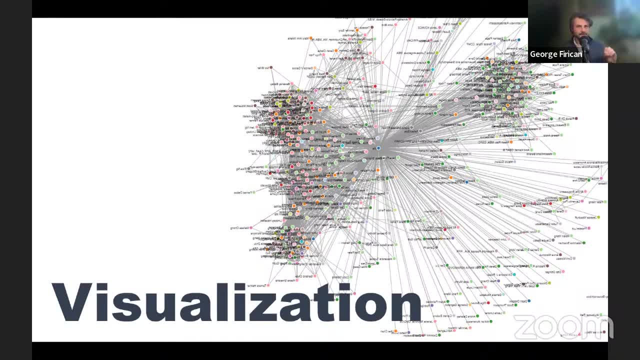 By the way, what we are seeing here is just a very small fraction of my LinkedIn connections And, uh, I don't think you can distinguish any of them, but either way, it is public information And they're they're different clusters, are based on the different um professional relationships I've had with those individuals. 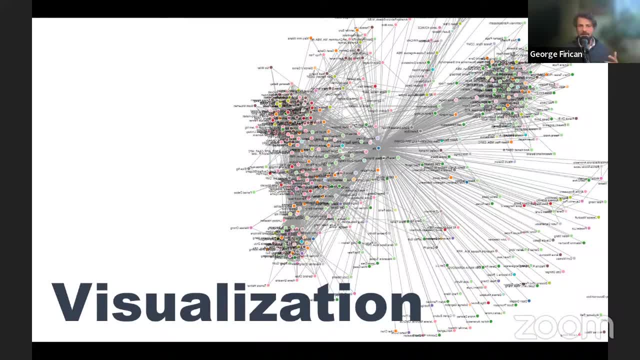 And there's definitely a lot of single ones, which are just mainly friends, I think. But again it poses that challenge: How can this be represented a lot better? And this is, like such a small fraction of my- I don't know- like 45,000 followers that I have. 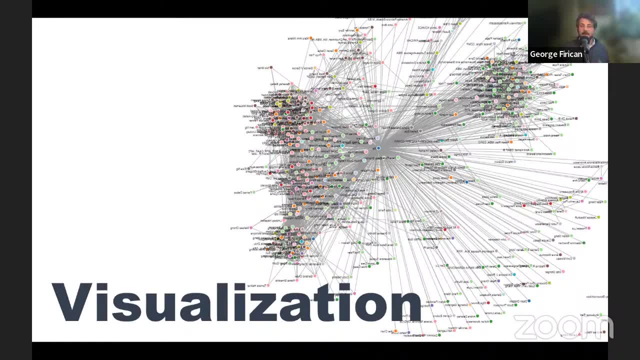 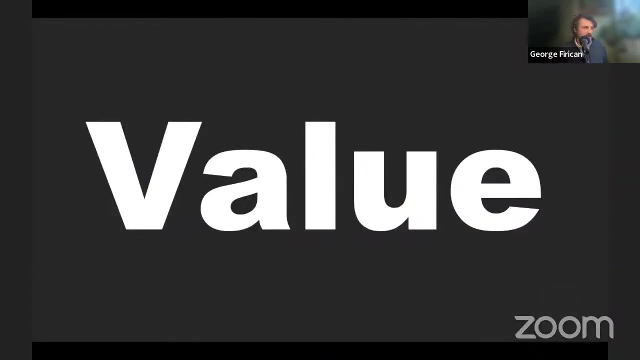 Now, combining this with, you know, the multiple Uh variables resulting from big data as a variety and velocity, and the complex relationship between them, we can see that developing a meaningful visualization, It's really it's not easy. Lastly, but arguably the most important V's of them all is value. 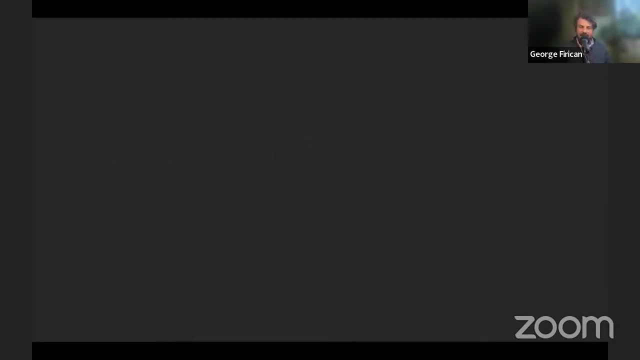 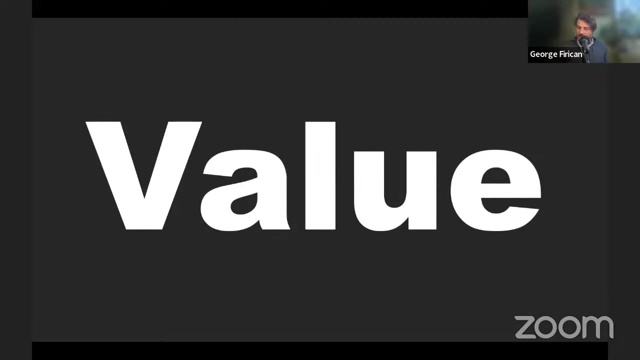 Big data is meaningless, Just nothing. There's nothing there If we don't derive value out of big data. So big data, I think it does bring a lot of value, So I want to share with you some examples on how that value comes, comes to be. how can we get that value out of our big data. the real world impact and value of big data. 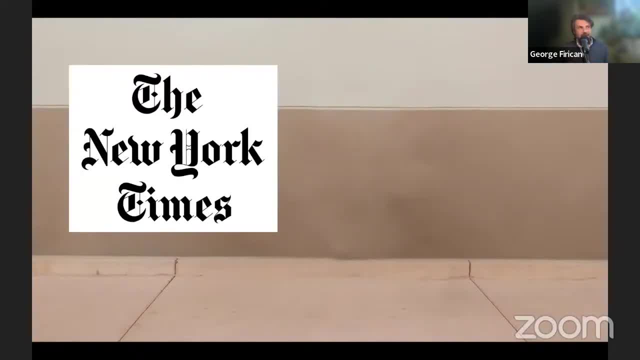 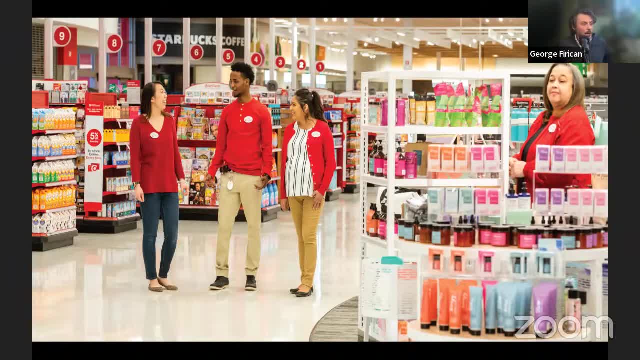 But here's the trick. There are, however, some brief periods in a person's life when all routines kind of just fall apart and buying habits are just suddenly in flux, And one of those moments is right around the birth of a child. Parents are exhausted, they're overwhelmed, and their shopping patterns and brand loyalties are. 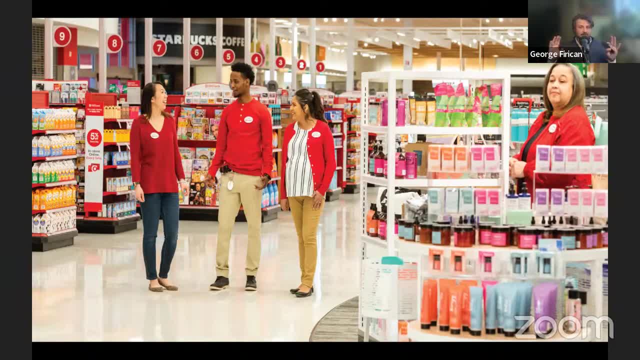 up for grabs. They don't care that they used to shop at that grocery store or they always used to get that brand. Oh, you know what. Whatever is most convenient, let me just grab that. I'm tired, I need to get home, And I'm not speaking from experience, but from everybody that I'm seeing. 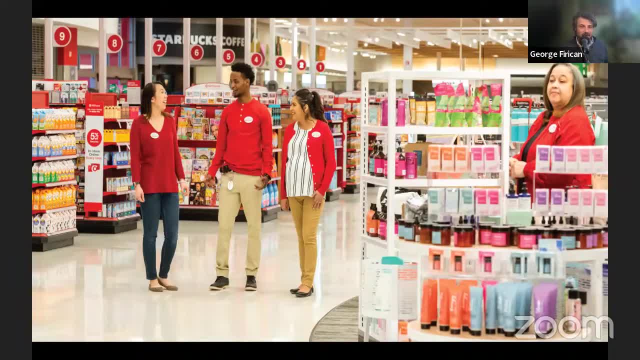 across and near me that have kids. that's kind of really how it is. So, yes, their brand loyalties, their shopping patterns, Everything it's up for grabs now, during those times. But timing is everything, because birth records are usually public, at least in the US, The moment a couple is having a new baby. 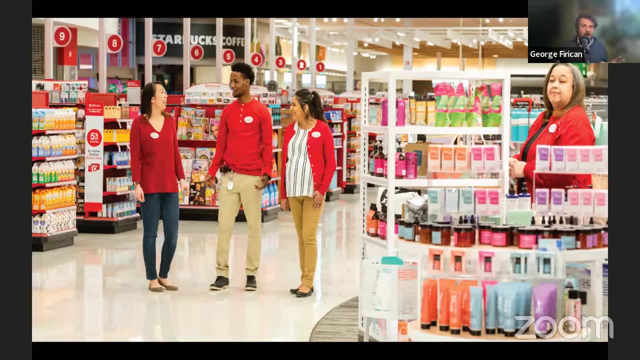 they're almost instantaneously just barraged with offers and incentives and advertisements from all sorts of companies, which means that the key here is to reach them earlier, Before any other retailers. no, You know that a baby's on the way for you know, this couple, this person, whoever's having the 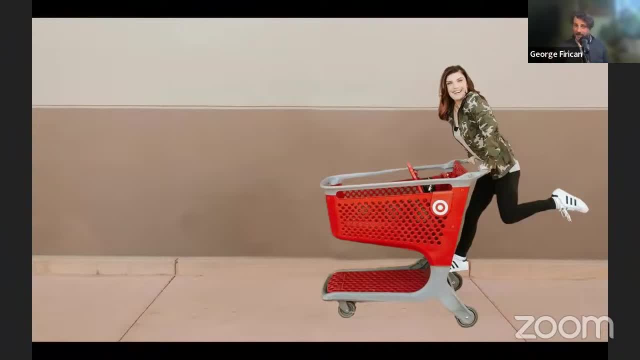 baby. So this was Target's challenge And Target studied consumer purchase patterns and they kind of knew that certain purchases like zinc and iron in large quantities and cocoa butter lotions kind of signal that a child will be on the way And Target's level of confidence in this model. 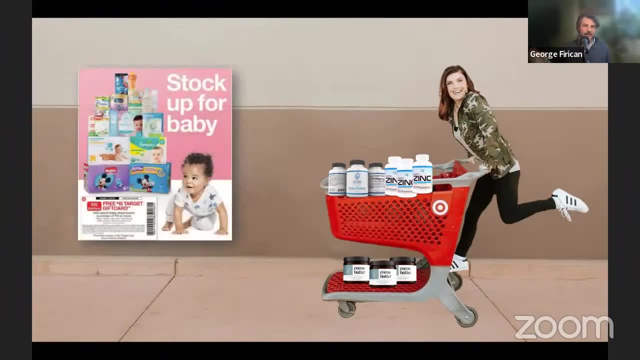 was just so high that it sent this- you know mailer to the young lady, to the 16-year-old, offering pregnancy-related products, which really infuriated her father. at the time He complained loudly to a Target store manager, but later apologized after discovering that his 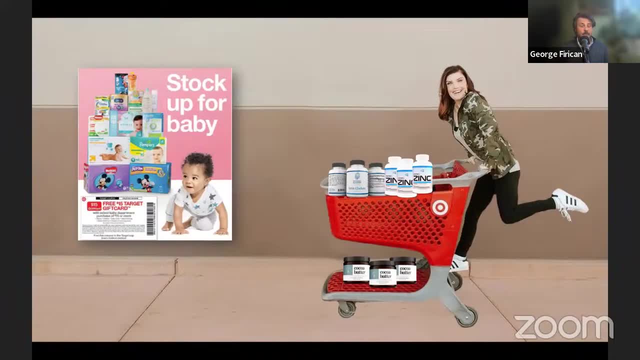 baby. his baby girl was, in fact, carrying her own baby. Yeah, As I mentioned vulnerability, that's definitely one of the big Vs. But Target well, there was a lot of value in finding out this information and finding out, well, who's going to be your parent in the next few months. Let's 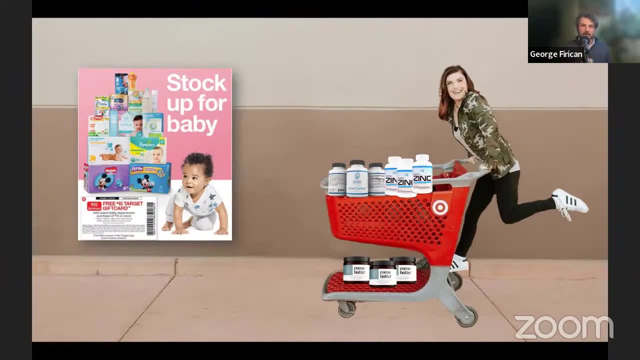 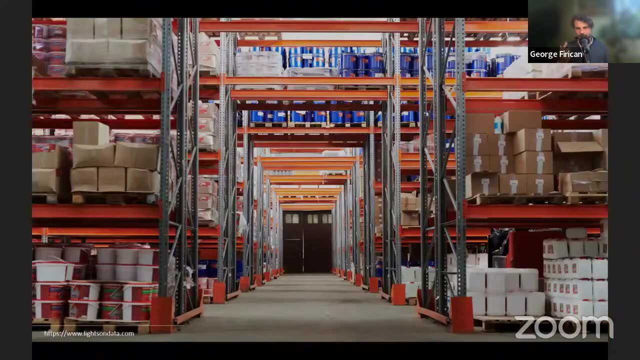 Target them. Let's get them loyal to our brand. Let's show them that they can get everything that they need from Target. Let's move away to the European continent now with the Vs. Let's take another example. This one is a European logistics company that operates more than 30. 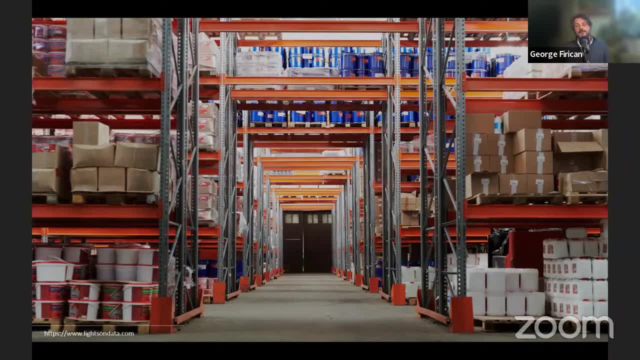 warehouses in Spain And they wanted to gain a deeper operational understanding of activity in its warehouses, in its- you know- facilities, in order to just sustain and increase productivity, ensure security of staff and goods and just optimize the processing of work orders. 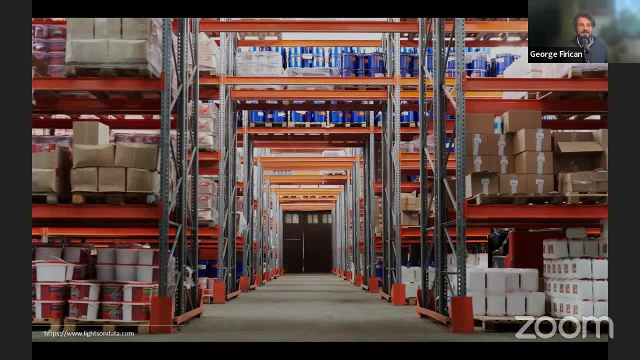 And, in general, that's what a lot of companies are trying to do right: Increase their revenue, decrease the cost, be more efficient. And well, they managed to do so by kind of tapping into this big data collected by their Wi-Fi infrastructure that they've set up in. 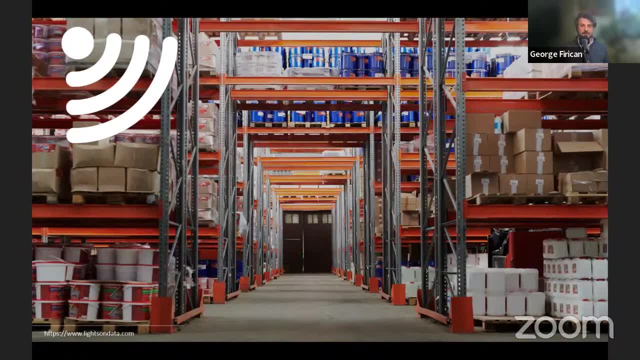 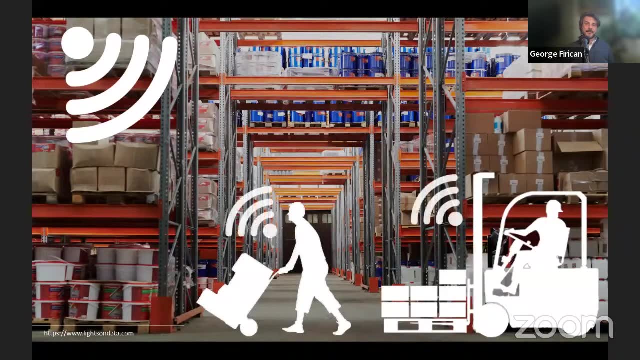 their warehouses And this Wi-Fi infrastructure was really collecting data related to devices attached to you know workers and equipment And that was constantly transmitting data and receiving it from the receivers there Among the warehouses, And they were collecting data such as you know device location and. 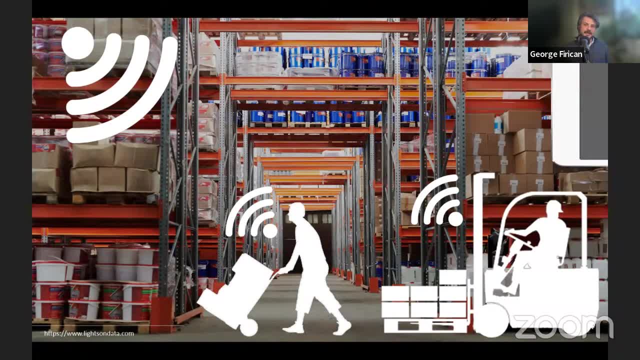 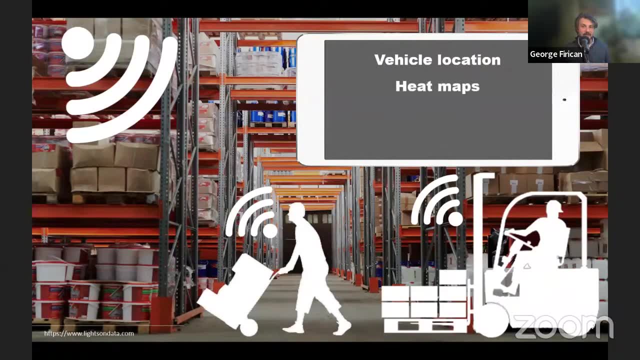 presence and motion, And tapping into this data really allowed them to know things such as the precise location of vehicles, as an example. you know what the population was in distinct areas and create some heat maps and flow maps viewed by time. It allowed them to see the heat maps and 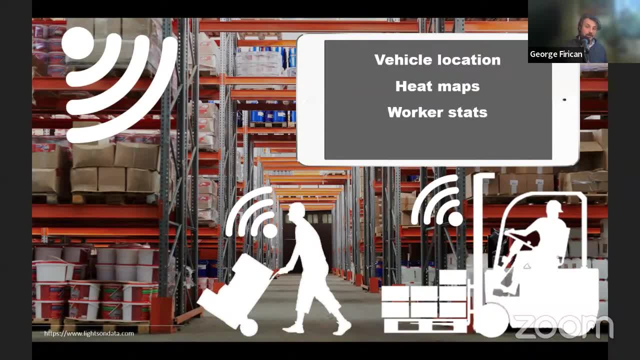 flow maps by device As well by vehicle, specific zones and so on, As well as the worker arrival, worker departure, even when people were taking breaks. I know it sounds a bit spooky, but you know they were obviously gained their workers permission to do this. I guess it was in the contract or something. 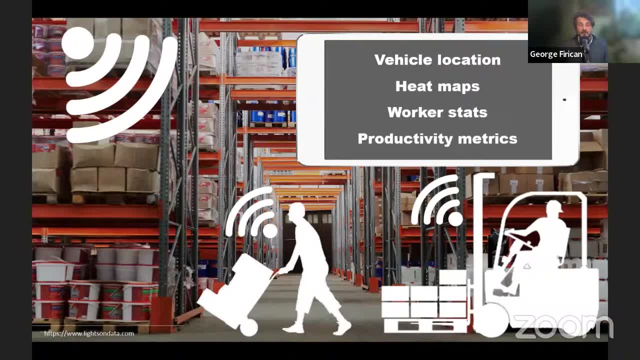 And productivity metrics, you know, such as the time between different operations. Crazy stuff, Big data. for sure, in terms of the Wi-Fi signals, there The complexity was more into the project, or not? Well, how do you kind of make meaning? 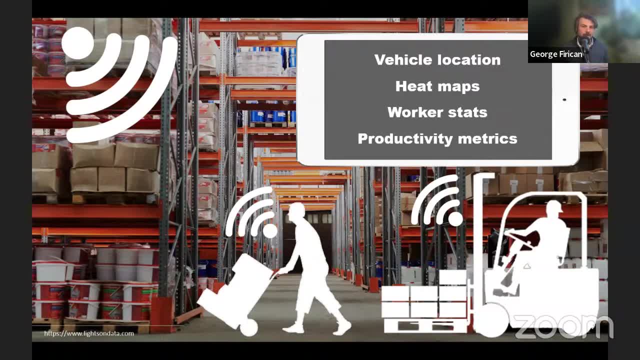 out of it? How do you get that value out of it? And they were able to, you know, get all these different stats and all this information. that then allowed them to kind of see what works, what doesn't, where efficiencies are needed, what can be done to be improved and how they can just 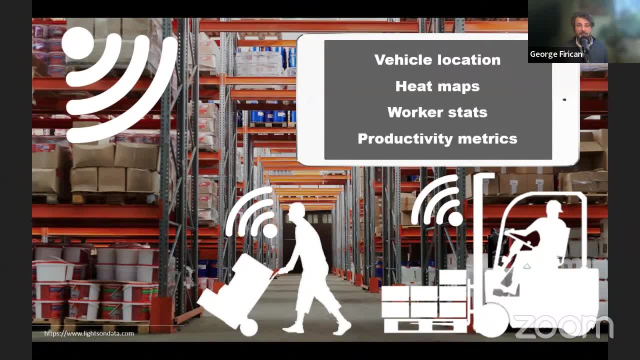 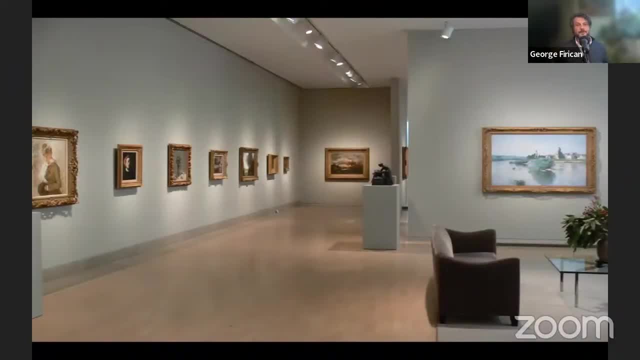 optimize their processes overall, And it really really helped them out quite, quite a bit. Let's take another mental trip, This time around to the Dallas Museum of Art. I think it was in January 2013.. The museum kind of launched a goal to implement data-driven. 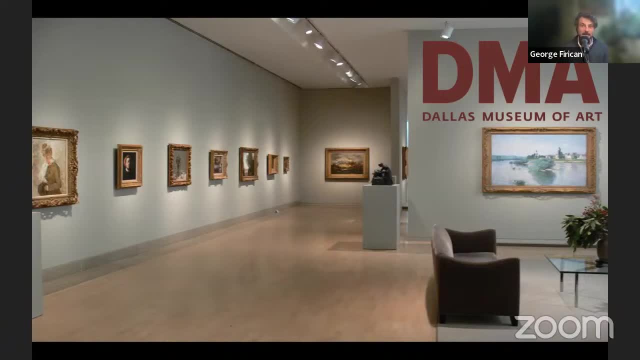 management within their organization, attract new customers, involve customers and foster customer loyalty. Okay, how are they going to do that? Well, they started by offering free membership in return for capturing their data, their members' data, So guests could now use their smartphones to kind. 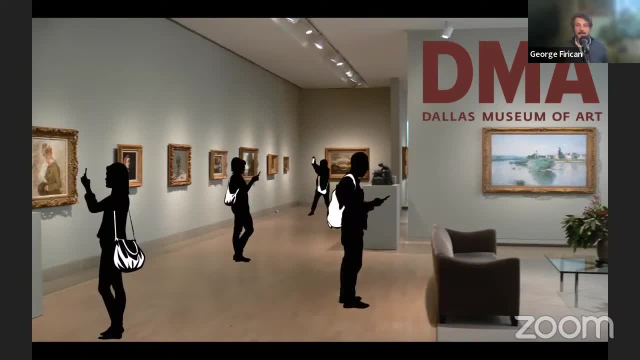 of check into the various spots And they would just interact with the pieces of art. Plus, the museum could actually track where and how they were going and walking through the museum- By accessing the museum app, I guess, and agreeing for all of this to be tracked And, in exchange, 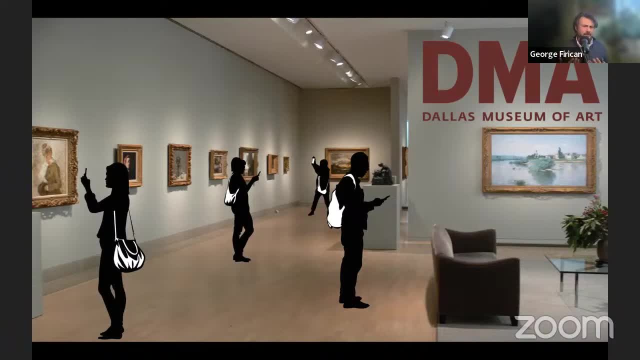 because there is usually an exchange that happens. you know why would I give you my information? for what? Well, you know, they would accumulate points that they could redeem towards various rewards, such as maybe some free museum lectures or some special events like after-hour events. 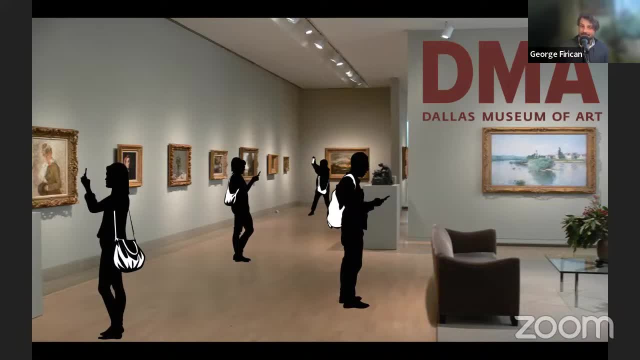 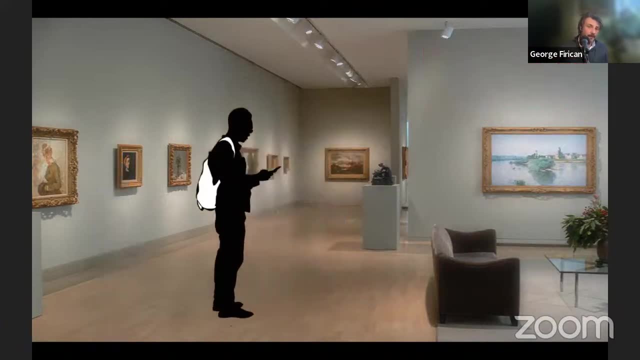 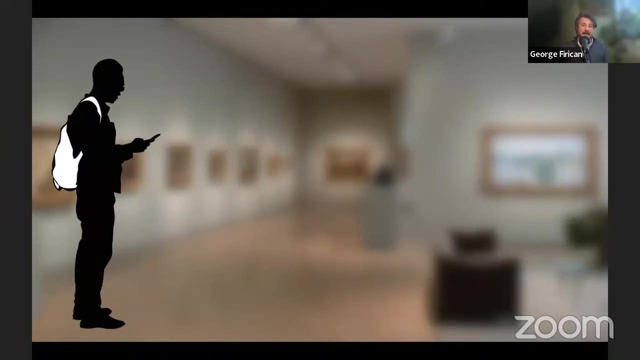 you know, special exhibitions, free parking, Maybe some gift shop discounts, So there was definitely an incentive there that was given to their members. The cool thing is that because of this they had 100,000 new members being added in- I think about a year and a bit a year and like three, four months And 40% recurring visitors. 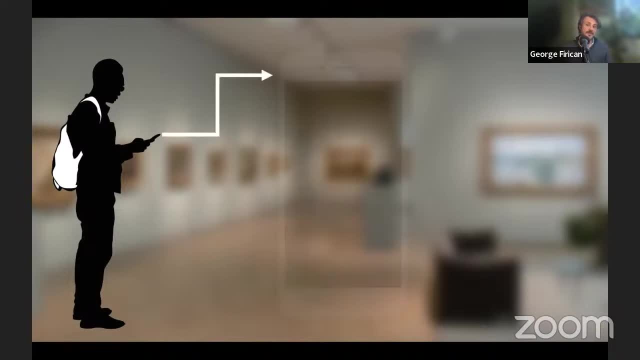 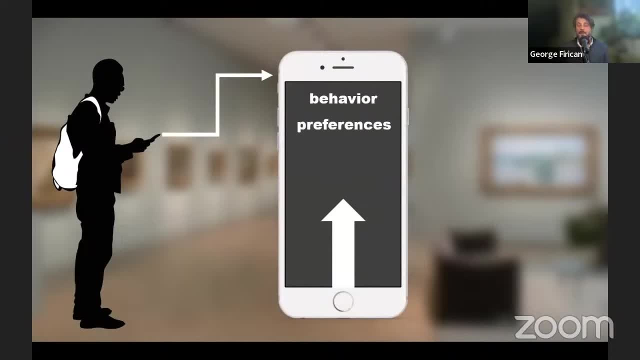 were able to get a lot of new members, And so they were able to get a lot of new members, And so they behavior and preferences. you know where visitors were from and just how often they were visiting a lot of cool stuff. Additionally, more visitors to this museum was really translating into more. 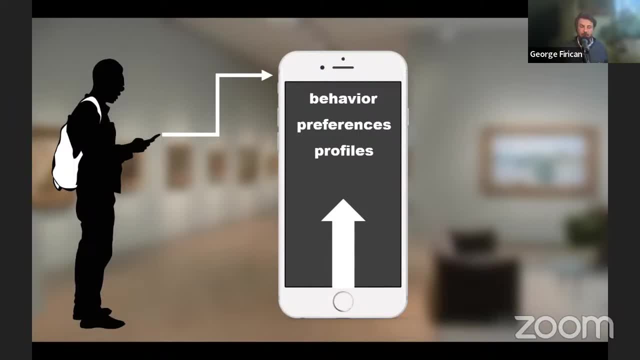 revenue in other areas. So, even though the museum was now offering free membership- you did not need to pay to get into the museum if you were a member, and you could be a member for free in exchange for your data- the revenue still increased. 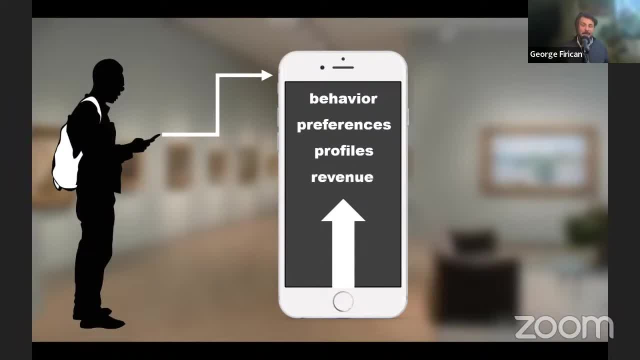 Well, why? Because they had so much more food traffic. now, You know, they had an increase in sales for their retail store, and even parking Parking was, you know, charging, and they were actually making quite a bit of money out of it. 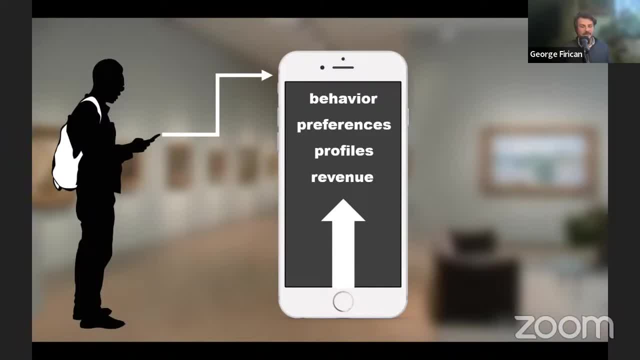 There was a bit of a downside- and this is, you know, overall, because other museums kind of adopted a similar trend. The downside that I think they had to, you know, just keep an eye on was the fact that it could lead towards producing a museum experience. 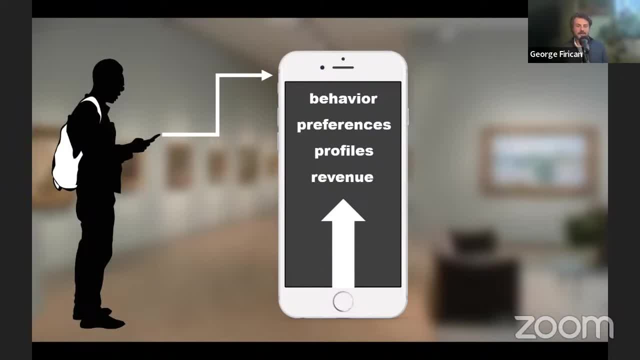 in that kind of pleasing the crowd. So just putting artifacts in there that were attracting the crowd for the sake of attracting the crowd and getting all this information, they would know, okay, what's an interesting piece that we can put on there. that is really, really, you know. 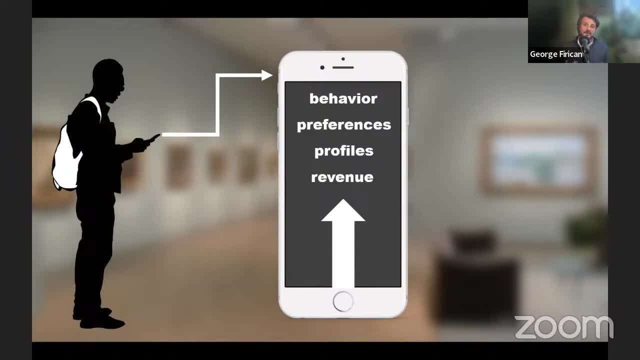 interesting to our crowd And not necessarily focusing on historically or artistically significant exhibits. So sometimes things are very important from a historical artistic point of view, but maybe it's kind of not the right time to show it. I don't know. 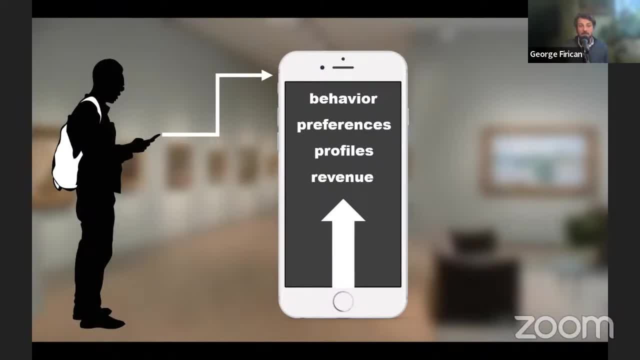 Of course, security and privacy is, you know, also a big risk. You are collecting all that information on the members, on the visitors. You definitely don't want that to be leaked in any way or be used in an unethical fashion. The cool thing is. 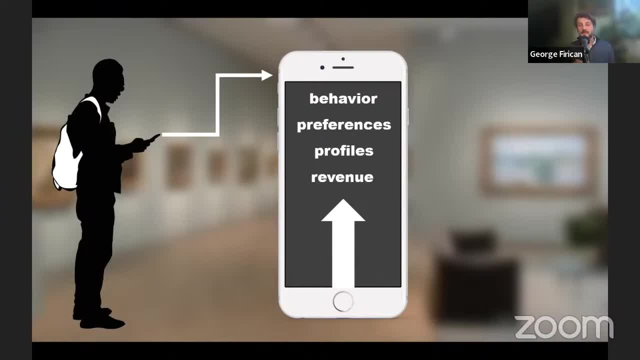 thing, though, is that it also makes more convincing appeals to potential sponsors, to things like museums. you know, uh, certain, uh certain data collected from the re-arts program, like the dallas museum, would allow fundraisers to better tailor their communications and solicitations to their members, to their donors. so, for example, if you know that somebody was visiting every month. 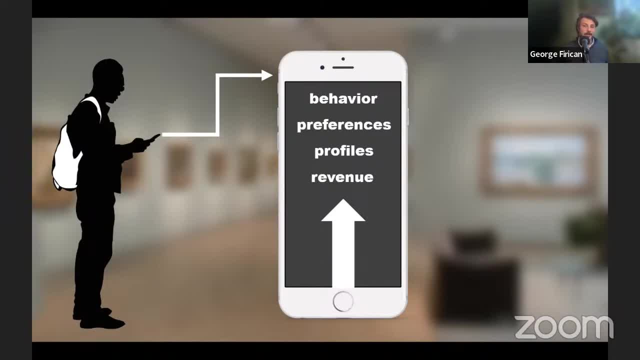 but has yet to contribute or to join the museum. you know you could tailor a special offer just for them, focusing on the benefits of that free admission, or give them a coupon for a free coffee at the museum cafe the next time they they visit. kind of is a thank you. 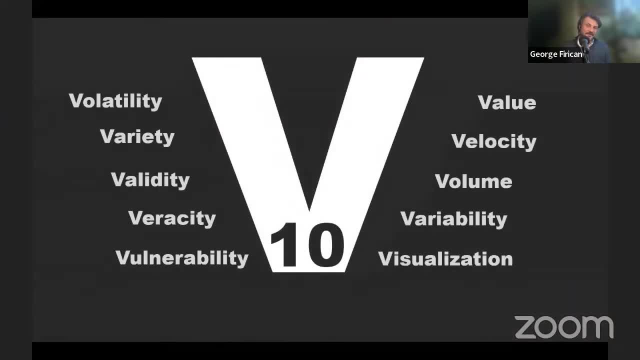 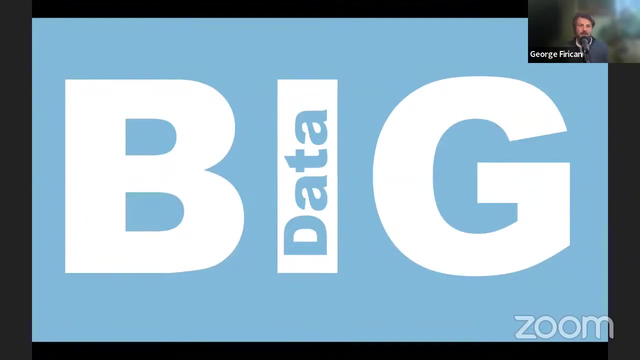 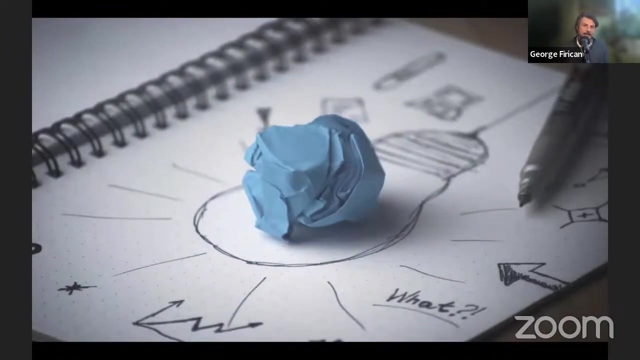 so big data, big data is quite complex and it's it's complex because, again, of these 10 v's which we covered. so when we think about big data, let's try and kind of throw the concept of big data out the window, because it's not the only important thing. data, big and small, medium size, all sizes. 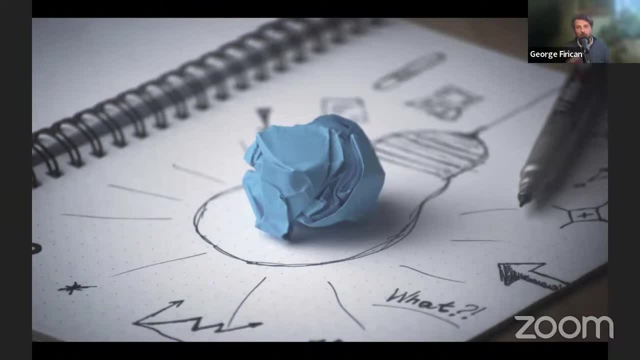 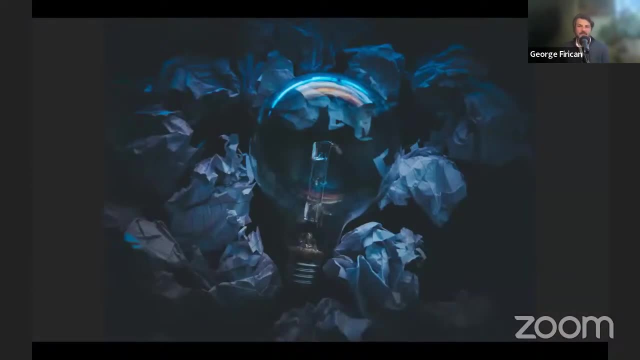 really possess complex problems which require innovative solutions. so i think that in many ways, that we all work with pieces of big data as we try to solve different levels of complex city. now we we all face issues maintaining the quality of our data, structuring it, classifying it. 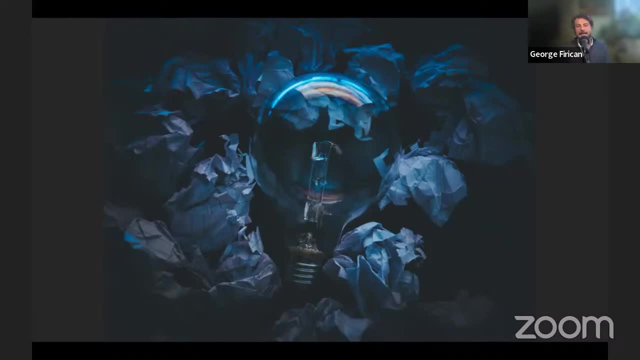 disseminating it and deriving information out of it and answering complex questions about it, and by being here today and attending, you know, all the different sessions that are free from the data science dojo. i hope that, uh, you know, you'll get a lot of lights on and have some aha. 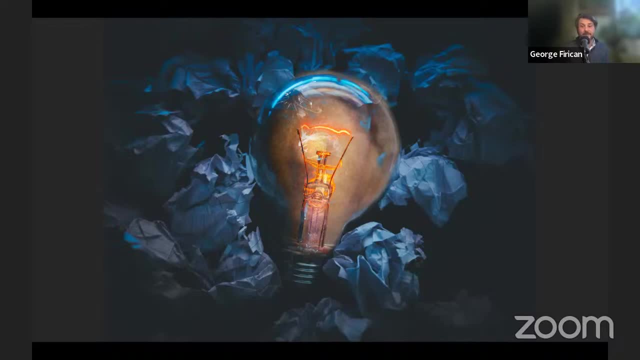 moments on how we can solve the data science dojo and how we can solve the data science dojo- the big problems with complex data. so thank you so much for having me. i look forward to chatting with you over one of the 2.2 billion coffees that are consumed today, so don't forget to get in touch. 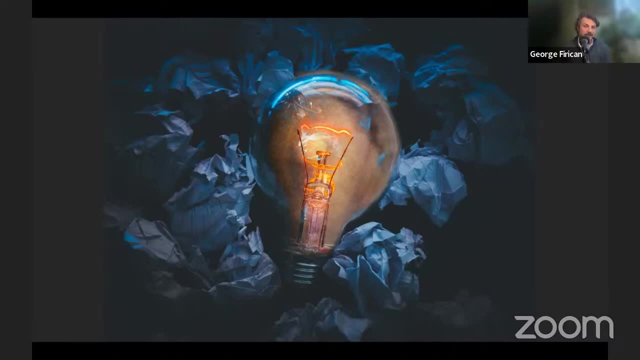 with me and, you know, connect with me on on linkedin, check out my lights on acom site, check out my youtube channel and i do always enjoy meeting new people in person or online and listening to your feedback, sharing ideas, information, so please don't be shy and get in touch. 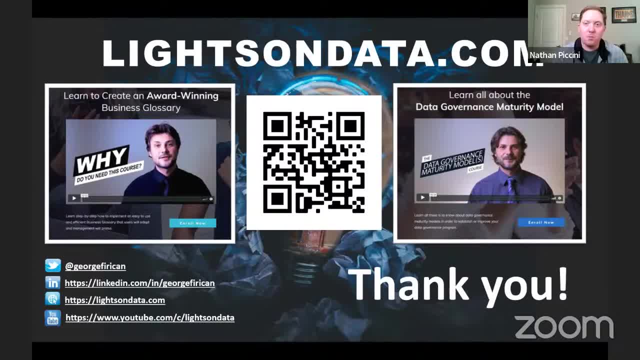 thank you. thank you, george, and is the is the best way for someone to get in touch with you through linkedin? is that the the best way that? yes, that's the preferred way. thank you, right. um, all right, george. thank you very much. um, we don't have any questions yet, but, um, i'm gonna steal a. 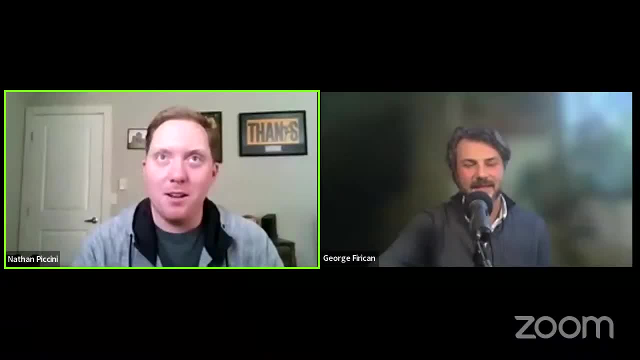 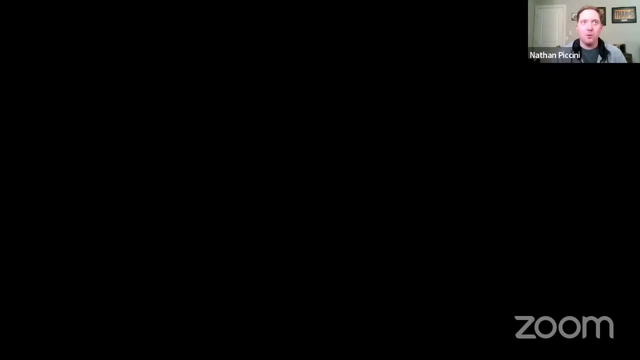 screen from you here really quick and then i'll have you bring this back up and and, uh, i'm sure that'll give people time to ask some um. so, uh, before we, um, you know, see if there's any final questions i do want to bring up: uh, next, next week, let's see. 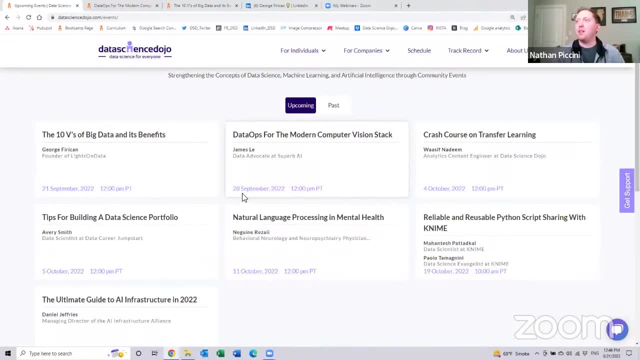 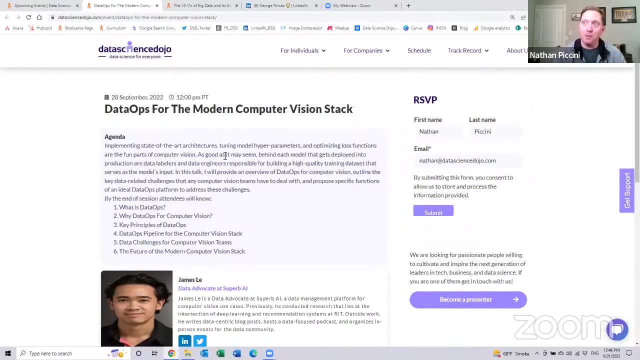 yep, so next week, uh, september 28th, uh, we have james lee and he's going to be presenting data ops for the modern computer vision stack and during this webinar, um, we're going to be talking about. what is data ops? what are some of the key principles? why data ops for computer vision? what? 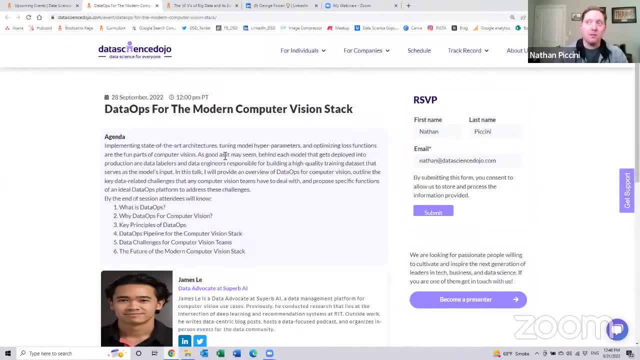 are some of the challenges and what are the challenges that you're going to be talking about. and you know what is the future of the modern computer vision stack, and and james is a data advocate at superb ai, which is a data management platform for computer vision. um, so, if you are, 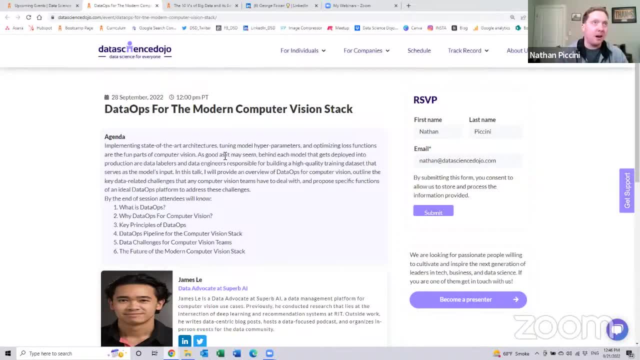 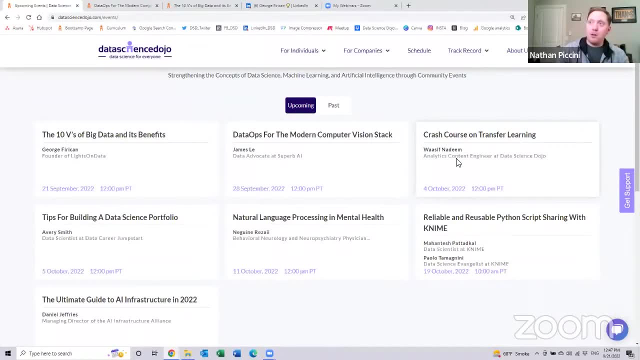 interested in computer vision in any way or data ops, i would suggest uh signing up for this event and giving it a look. we also have some good events coming up. in october we have a crash course on transfer learning, um tips for building a data science portfolio. so if you're trying to break, 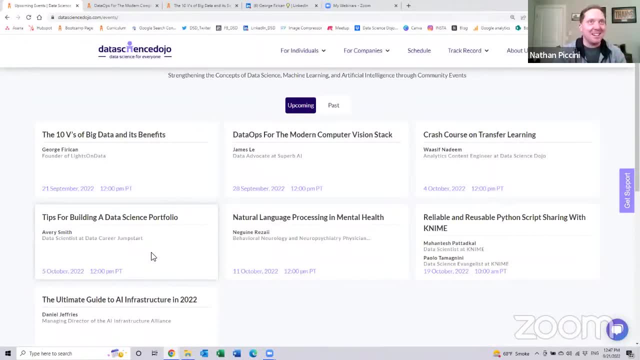 data science. you've probably heard that you need a data science portfolio. it's important for the job hunt, um. so october 5th with avery smith, the data scientist at the data career jump start, could be a good one for you to attend. um. all right, james, if you want to pull up that last. 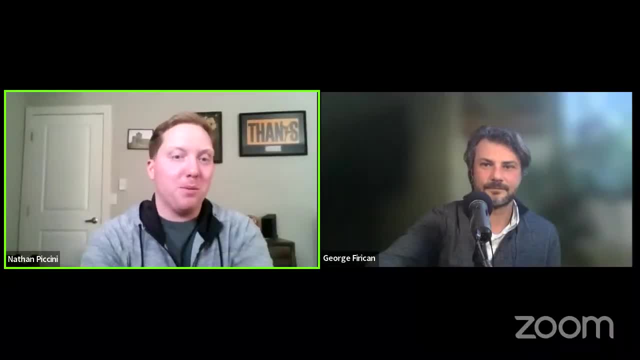 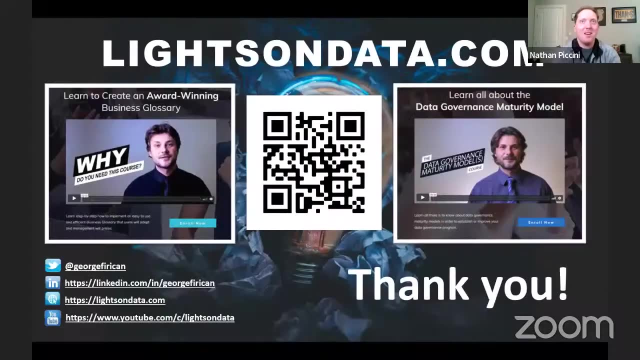 um, that last slide again. uh, give people a moment to uh, we can give them a chance to. you know, find you on linkedin, twitter and all those places as well. sounds good, and i do recommend, by the way, attending avery smith's um presentation. i, i know him, i'm lucky. 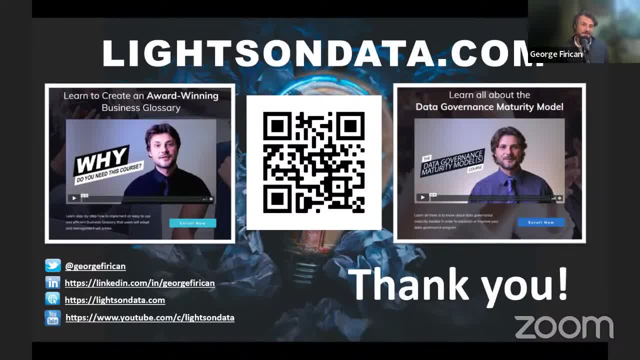 enough to know him and he has great content, so i'm looking forward to that one as well. i saw- i saw some of the comments uh on on what people thought of the, that grid of the. the satellite images were so uh. besides wheels of cheeses, i saw some seashells and clocks.